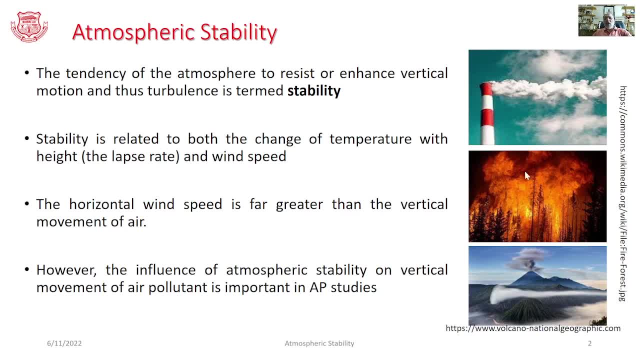 various pollutants. so in any of such, either man-made or natural sources, the behavior of the pollutant as it enters into the atmosphere will be solely dependent on this atmospheric stability. so the tendency of the atmosphere to resist or the enhance the vertical mixing and hence the existence of the 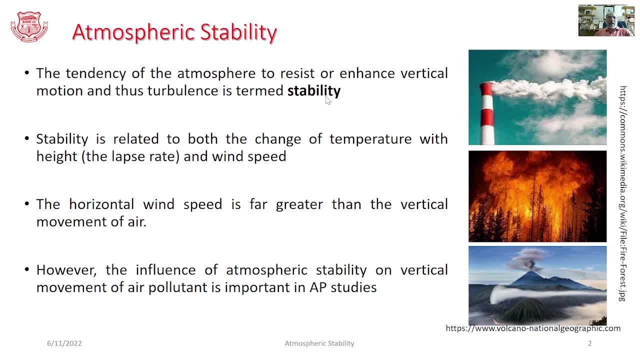 turbulence is termed as stability. as far as air pollution studies are concerned, you, this stability is related both with the change in temperature, as well as even the wind speed. the reduction or the increase in the vertical plane associated. the Earth's surface is also taken into account while determining the stability. 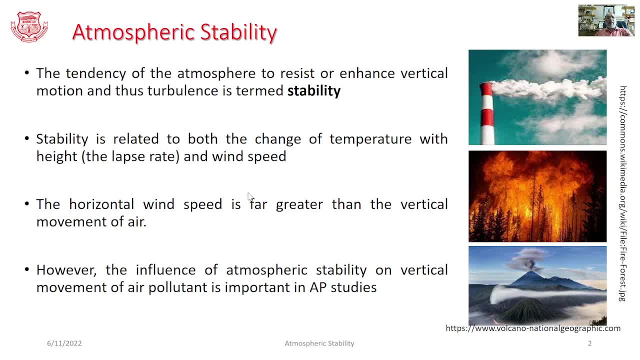 we know that horizontal wind speed is far greater than the vertical mixing that would be occurring in the atmosphere. however, the fate of the pollutant will be solely dependent on this vertical profile. hence, the influence of the atmospheric stability on the vertical movement of the air pollution is very important as far as air pollution studies are concerned. 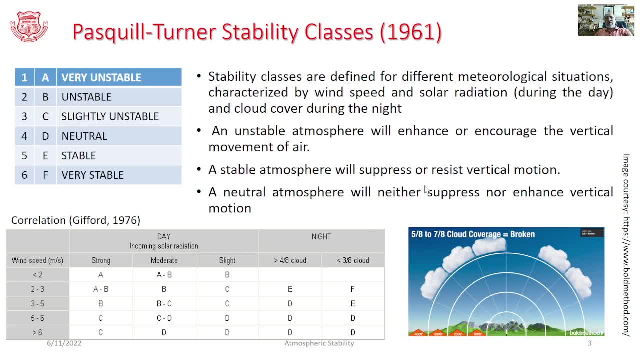 the one another. that is important to remember, that Pasteur's equation. so here, in the basis, the flow product ofласти might be好吃 xi. so, based on studies which are defining various stabilitic classes, say, for example, if we think of the national weather servicing station or national climatic centers, even there is one, Brookhaven- 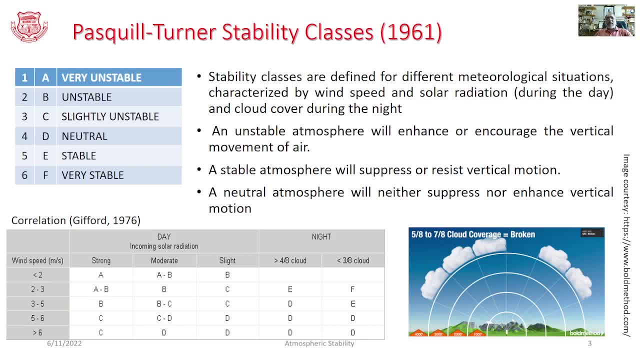 national laboratory. so all these particular agencies which are collecting the data associated with the meteorological parameters have attempted to give the various stability classes the possible terminal stability classes as were put up in 1961. the correlation among the various parameters is further given by Gifford and it is summarized in this particular table. 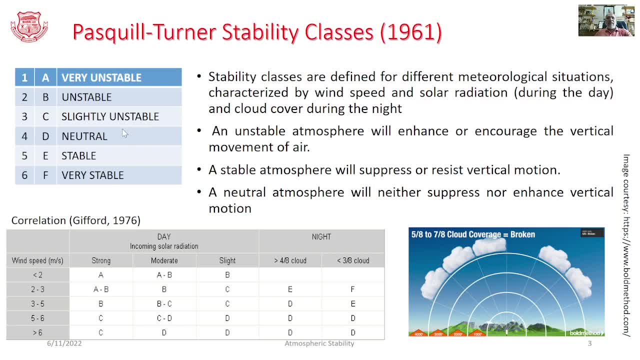 as you see, here, the stability classes are defined for different meteorological situations characterized by wind speed, incoming solar radiations and also the existing cloud cover. this classes are defined as a through f. this a is very unstable, b is unstable, c is slightly unstable, d is very unstable and e is unstable. so a is slightly unstable, b is unstable, c. 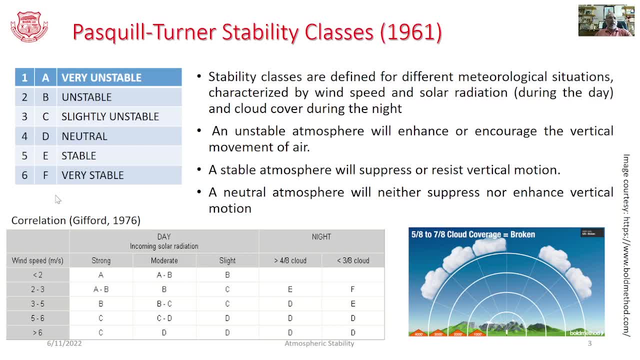 is slightly unstable, d is very unstable, that is a very unstable, a is very unstable, c is neutral, E is stable and F is very stable. As we move ahead, we will be able to focus and understand the meaning associated with each of these particulators. To start with, 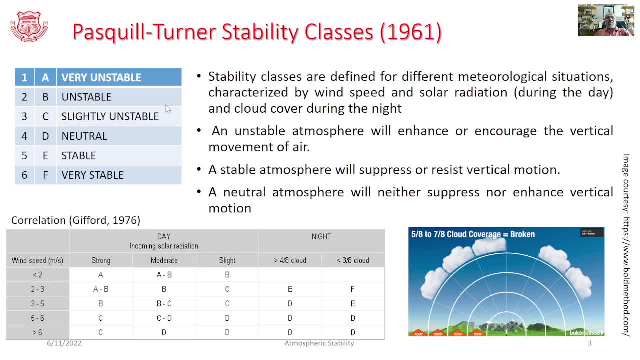 we will try to understand the meaning associated with the unstable. So this unstable atmosphere is to enhance or encourage the vertical mixing of the air, whereas this stable atmosphere will suppress or resist the vertical motion and the neutral atmosphere will neither suppress nor enhance the vertical mixing. So, as we try to understand the meaning associated with 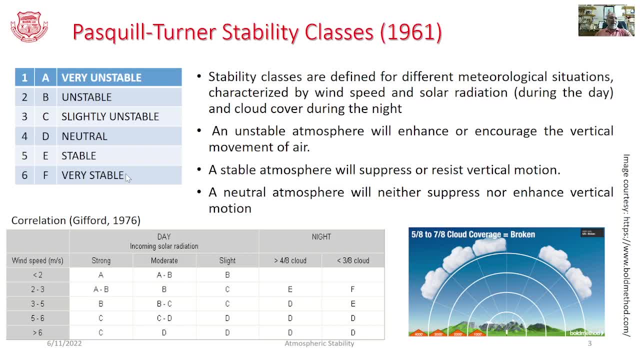 unstable, stable and neutral. understand very stable and unstable or slightly unstable is quite clear. one more thing that we have to think of: already we have discussed about the wind, so that particular wind speed and related characteristics already you know about. we have also discussed about the solar radiations associated. 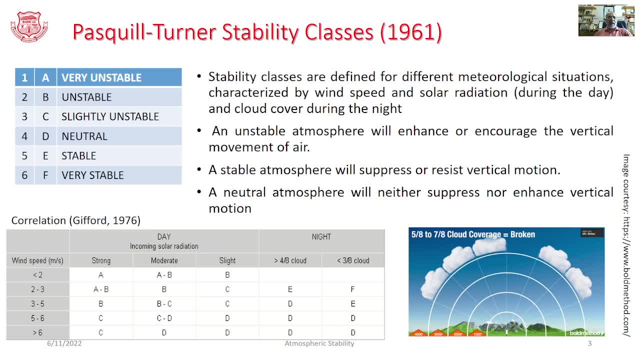 changes as far as earth's surface is concerned and also the related pollutant movements. so this strong say during the noon period say moderate, say noon to evening period, whereas early morning and the late evening will be giving about these slight solar radiations. as we consider this day time, we have to think of the relation as given by the g4, in terms 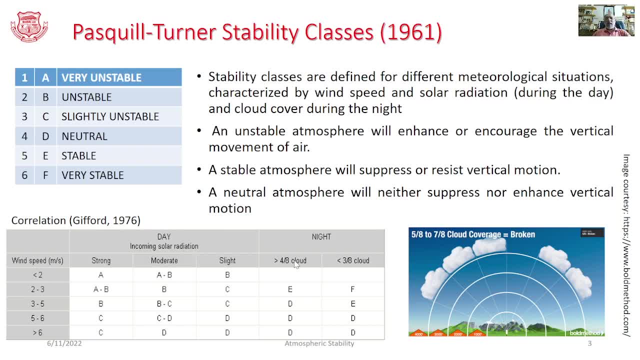 of these solar radiations. however, during the night, as you see, there will be the presence of the clouds. so here, the entire horizon will be divided into eight octaves and accordingly, here one the picture is telling us that some five octaves are covered out of eight. so, similarly, here as you, 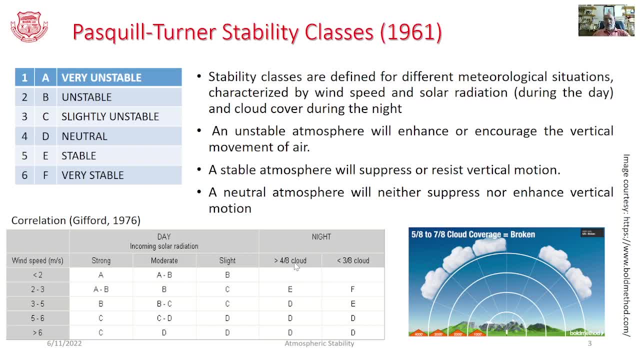 see during the night time if fifty percent of the cloud cover is there or if three by eight cloud cover is there. accordingly, here the situation can be considered in terms of that relevant class. so say, for example, if it is daytime and if it is noon, but if it is midday, so the temperature is Y Бог. 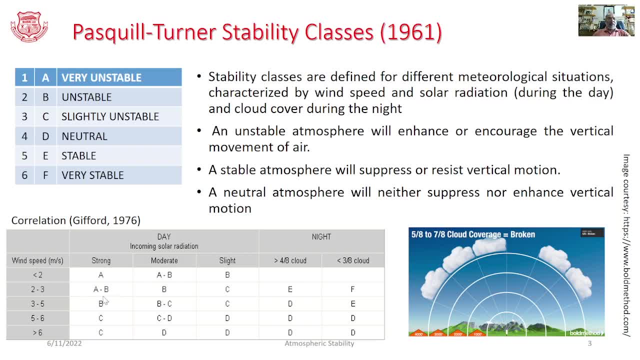 if the wind speed is ranging in between three to five meter per second, the class will be unstable, whereas, as we consider the incoming solar radiations, slight wind speed is higher than six meter per second. here the category is neutral. accordingly, even for these particular night periods- C, p and v, the temperature stillんで here stillenaˇs, the is for particular night periods, We can. 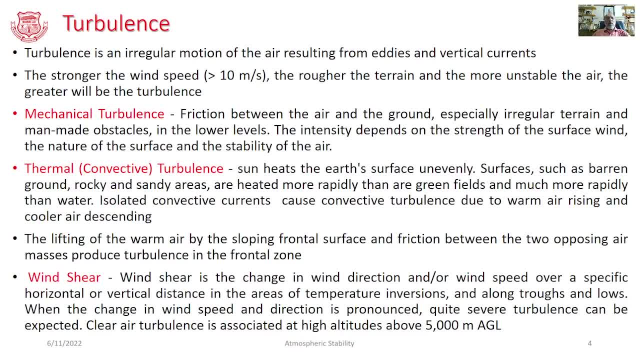 think of Now, while discussing about the stability we mentioned about this turbulence. So you already know that this is irregular motion of the air which is resulting from the eddies or the vertical currents. again, that would be related to be the incoming solar radiations, that geographic location as 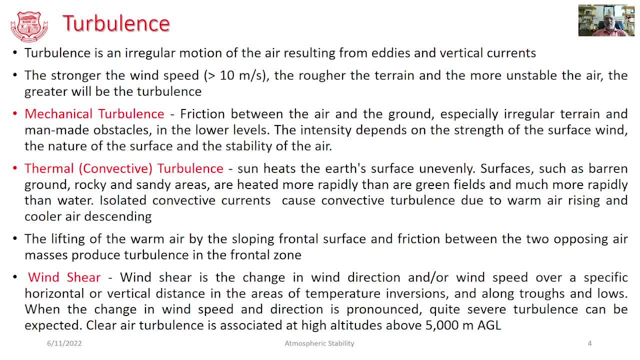 well as the daytime or evening time, or even the season, the local terrain and some such happenings. So the stronger field speed, which is stated to be greater than 10 meter per second, will be associated with the rough terrain and hence there will be more unstable the atmosphere. Hence, as we consider this stronger wind speed rougher, 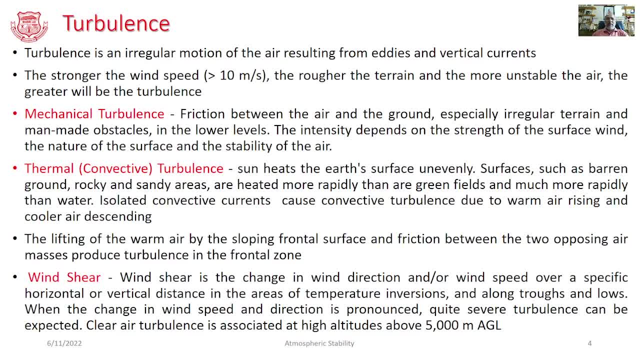 terrain or more unstable air, it will be associated with the turbulence in positive manner. Let us also get introduced with the mechanical turbulence, thermal turbulence and the difference in that, So as the wind moves across and over the ground surfaces, so as it moves, especially during any period, over the 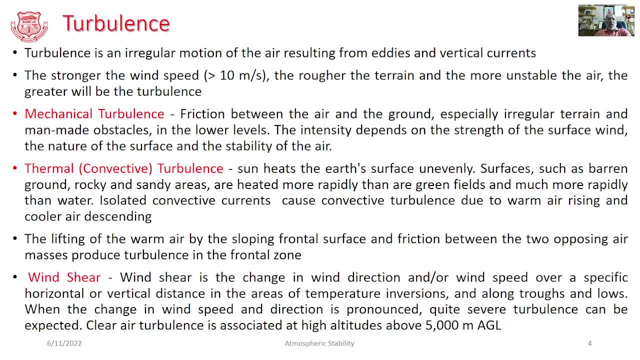 irregular terrain and the man-made obstacles, there will be friction. This friction is termed in terms of mechanical turbulence. Its intensity will depend on the strength of the surface, wind, as well as the nature of the surface and the stability of the air. As we discussed about the solar radiations, as they reach the earth surface, they will 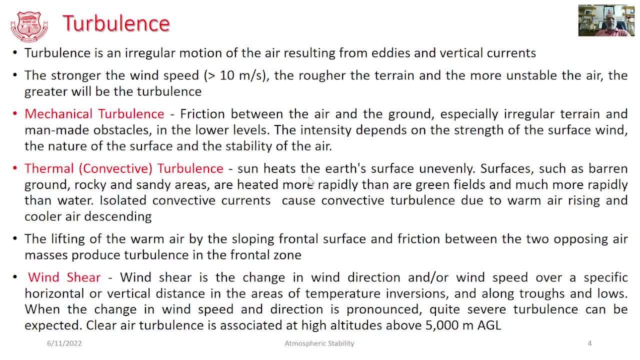 be hitting the various zones in the different manner so accordingly, there will be development of this thermal turbulence. So, as we discussed about certain local phenomena such as barren ground or rock and sandy terrains, they are heated more rapidly as compared to water bodies, as well as even the greenfields. 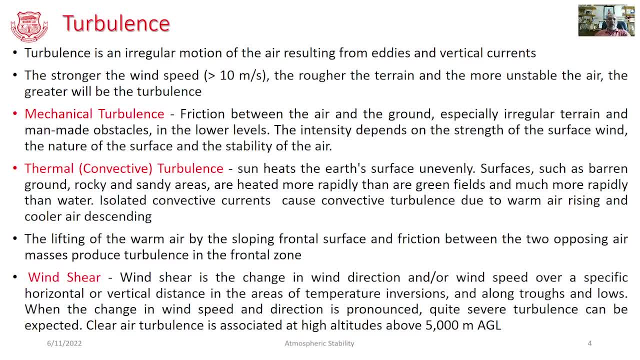 and hence will be development of this thermal turbulence in varied manner. These isolated convective currents cause the convective turbulence due to the warm air rising and also the cooler air that is descending. Also the lifting of the warm air by sloping frontal surface and the friction between the 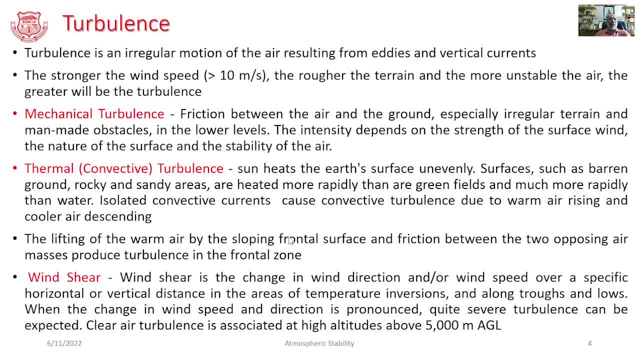 two opposite air masses. as we discussed about the cold fronts or hot fronts, they produce the turbulence in the frontal zone. This wind shear is the change in the wind direction and the wind speed over the specific horizontal as well as the vertical distances in the areas of the temperature inversions. 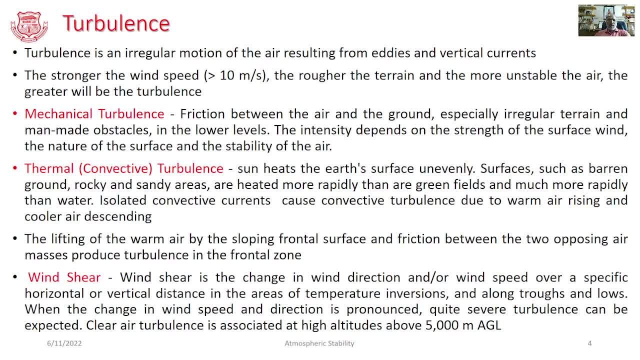 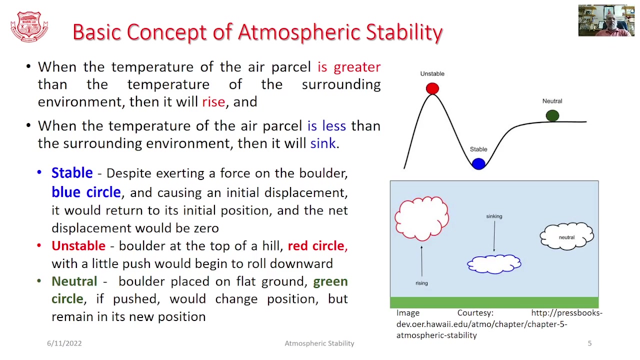 and along the troughs and loads. when this effect is pronounced, there will be severe turbulence. this clear air turbulence is associated at high altitudes above the 5000 meter, as it is considered average ground level. so, having understood the terms and the exact meaning associated with the 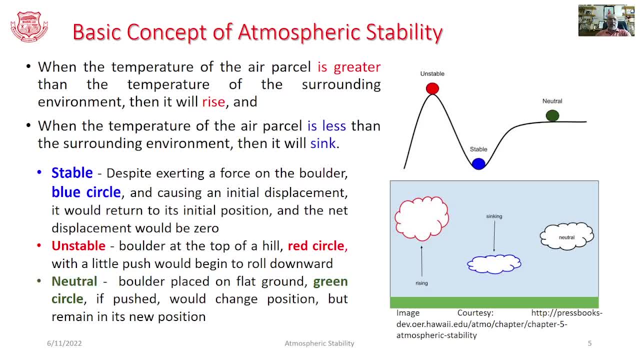 turbulence. let's come back to atmospheric stability. so we discuss about this particular atmospheric stability as the tendency of the atmosphere allowing the vertical mix it. now let's consider one more terminology, that is, air parcel. this term, air parcel, is telling us about the specific volume of air. 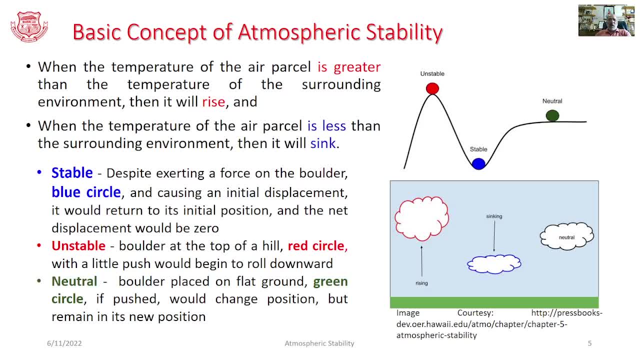 which will be having very similar characteristic as that of the atmosphere. however, we can attach all the dynamic as well as thermodynamic properties to that parcel. it will be having enough number of the air molecules, but it won't be mixing with the surrounding atmosphere, so this is sort of theoretical approach. 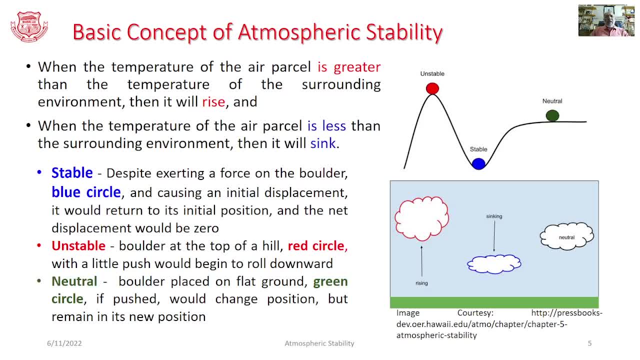 this air parcel does not have any specific shape. however, it will be maintaining its characteristics and its own. so as such air parcel enters the atmosphere, if its temperature is greater than the temperature of the surrounding, it will keep on rising with height. however, if the temperature of the atmosphere increases more and more than the temperature of water, it will gain more air volume. then its temperature will rise further with that temperature for sure. 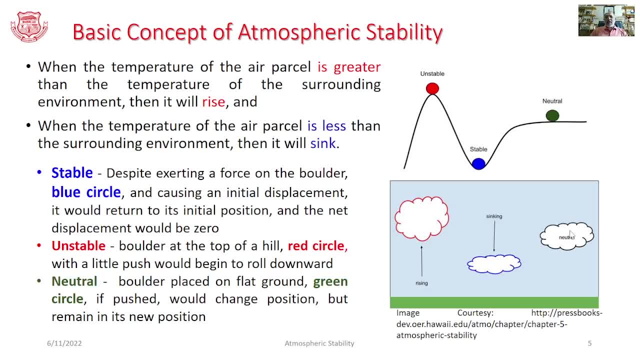 emitted air parcel is less than the surroundings, it will be sinking. If the temperature of the air parcel and if the surrounding atmosphere has got the same temperature, the air parcel will be moved according to our intention or the way it is moved. it will be remaining stationary, So this particular thing can be. 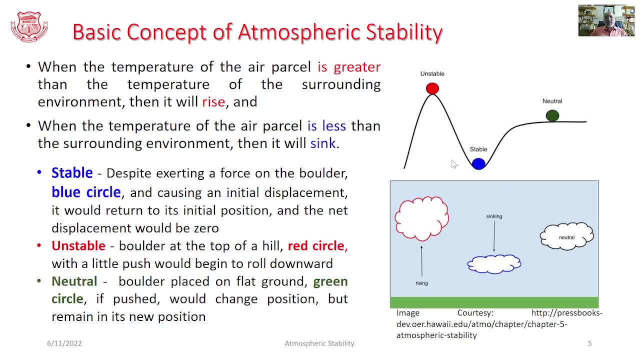 considered with this particular analogy Here. as you see, this is trough like portion. so if we consider certain boulder which is at the end here, even if it is moved by exerting certain force, it will come back and it will be remaining as it is. it indicates its stable nature. However, as we consider, 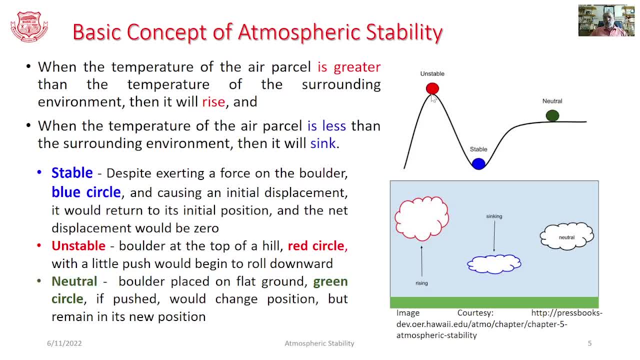 this say ridge like portion here. this boulder which is at the peak, if provided with some force it will simply descend down the slope and it will be accelerating. It indicates the unstable nature of the atmosphere. If we consider the horizontal surface, the boulder which is resting here, if applied with 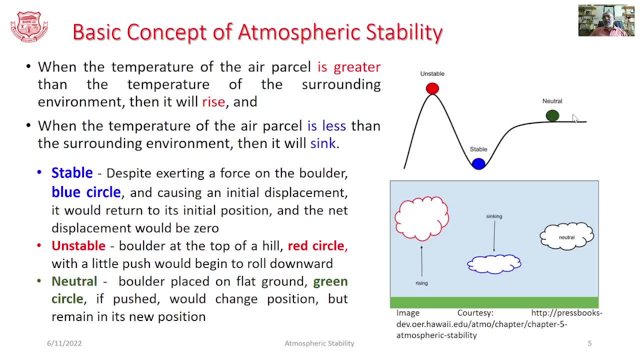 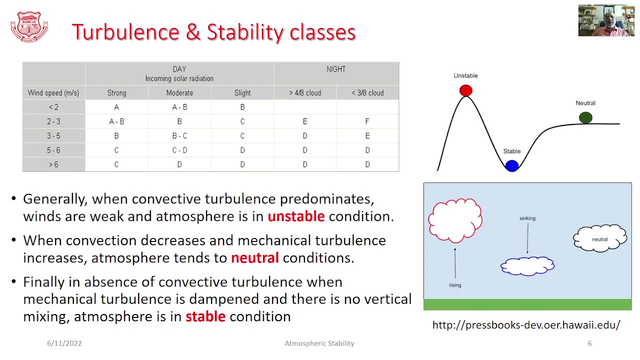 certain force, it will keep on moving till the force lasts. As the force becomes zero, it will be remaining as it is at that particular place and hence it indicates the neutral stability. So, coming back to again the past question, As you have understood the meaning associated with the solar radiations, the cloud cover, 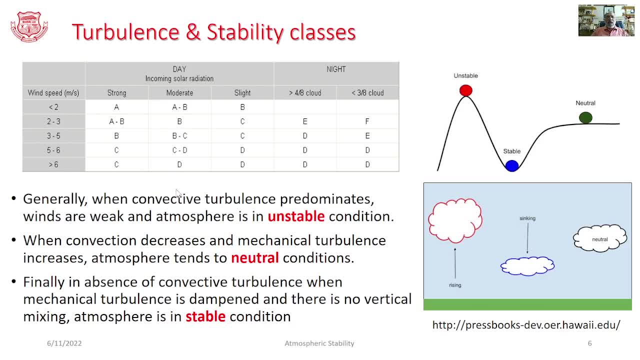 and wind speed and associated classes. Also, you got acquainted with the terms unstable, stable, neutral and their rising up or sinking down or remaining neutral, and also the meaning associated with the turbulence. So when convective turbulence predominates, the winds are weak and atmosphere is said. 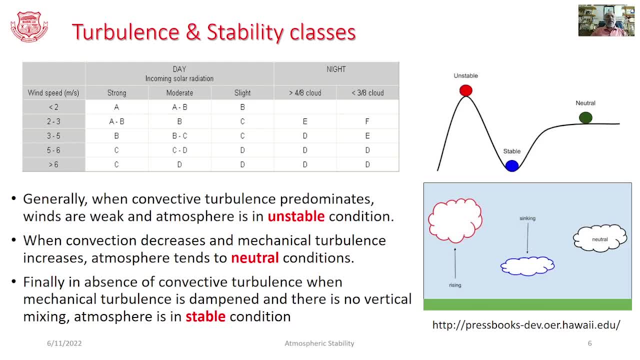 to be unstable When the convection decreases and if the obstacles are more. hence the mechanical turbulence is more, And under such circumstances the wind speed is also unstable. So when the convection decreases, the wind speed is also unstable. So when the convection decreases, the wind speed is also unstable. 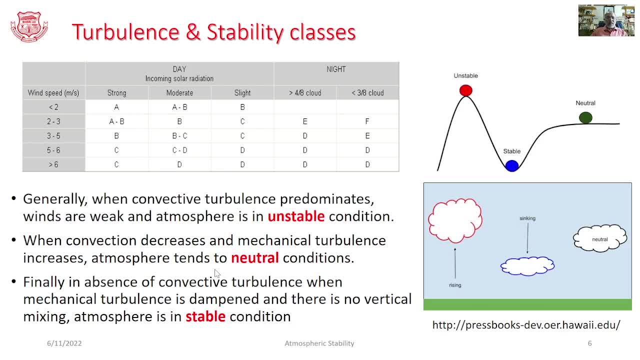 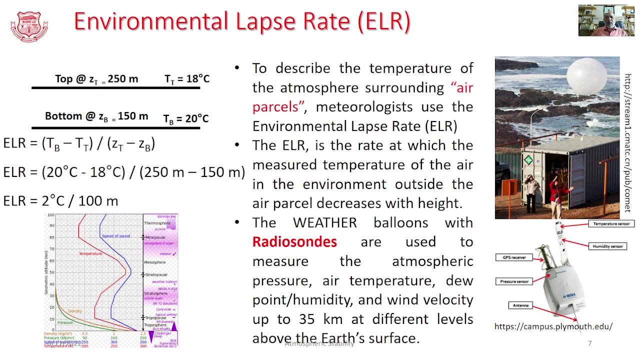 In the absence of this convective turbulence, and if the effect of the mechanical turbulence is not much, the vertical mixing won't be much, and hence the atmosphere is in stable condition. Now let us try to understand the meaning of lapse rate. So the first thing is already you got acquainted with this air parcel. 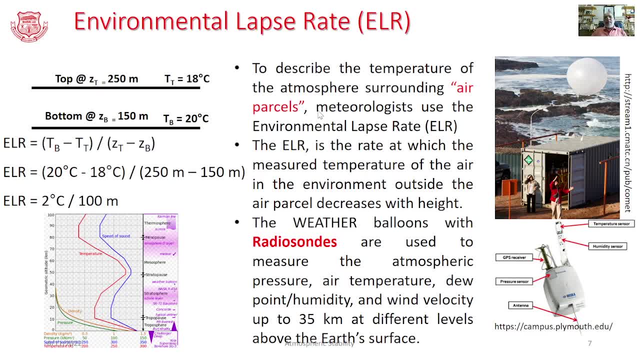 So we have to compare now the temperature of this air parcel with its surrounding And in order to have that particular temperature profile of the surrounding, we make use of the term environmental lapse rate. This lapse rate is similar rate at which the major temperature of the air in the environment outside the air parcel is equal to the temperature of the air parcel. 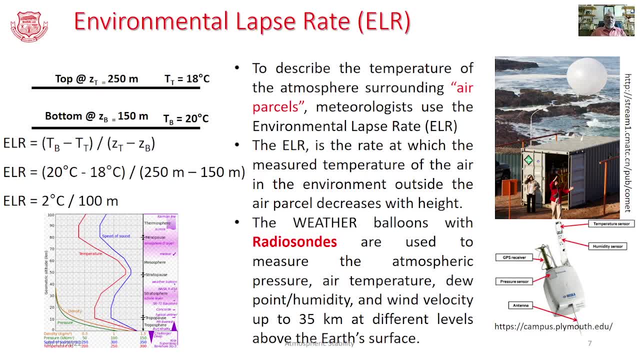 The temperature of the air parcel decreases with the height. So, as we consider this particular case, at certain height of this 150 meter the temperature is of 20 degree centigrade. After 100 meters, the temperature is of 18 degree centigrade. Hence there is a lapse of 2 degree centigrade that is occurring over the 100 meters. 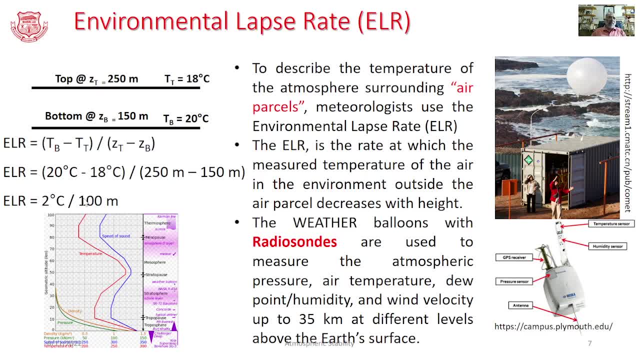 Hence this lapse rate, or environmental lapse rate, is of 2 degree centigrade per 100 meters. This lapse rate can be easily determined by making use of these wither balloons. So these wither balloons are equipped with the radio sounds which are used to measure the atmospheric pressure, air temperature, dew point, as well as the humidity and even the wind velocity, up to 35 kilometers at different level above the earth's surface. 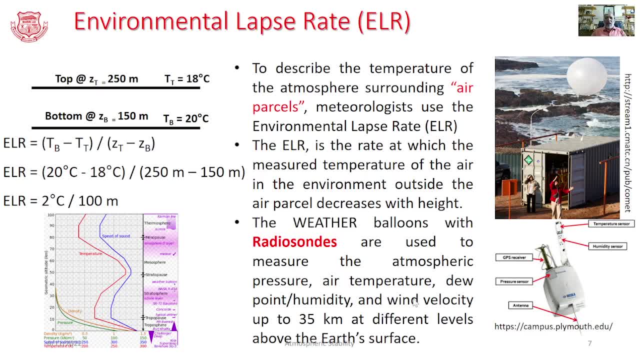 As we plot the temperature of the air parcel, As we plot the various parameters that have been monitored at a place can be plotted in this manner, and the plot is termed as sound gates. So this is a particular picture which is indicating the launching of the balloon which is equipped with these radio sounds. 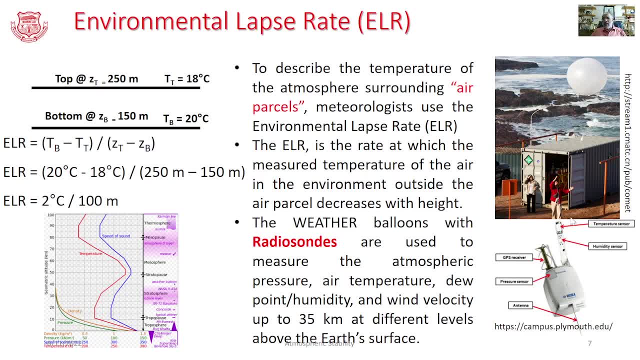 And this radio sound is equipped with these variety of the sensors meant for humidity, temperature. It is also giving a particular location through the GPS receiver, as well, as it will be giving the pressure sensor and even it will be having. it has some antenna. 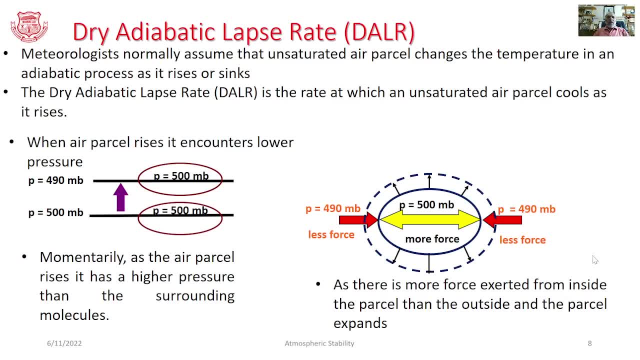 The second app is the radio sound gate. The second approach associated with this lapse rate is dry adiabatic lapse rate, So as the air parcel moves through the vertical profile And if the air parcel is unsaturated It will be termed to be dry. 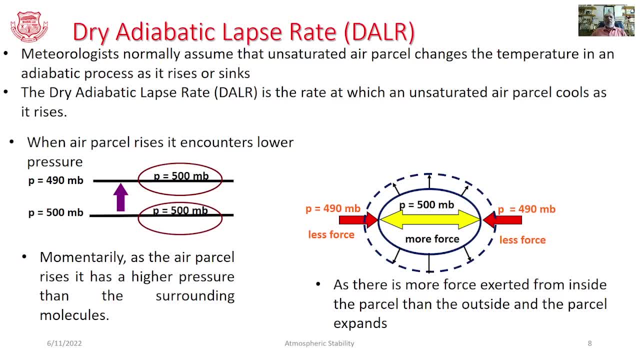 As it moves and as it changes its temperature, As it rises or sinks, There won't be any exchange of the energy with the surrounding atmosphere. Hence the term adiabatic. So as we consider all such situations, There would be dry adiabatic lapse rate. 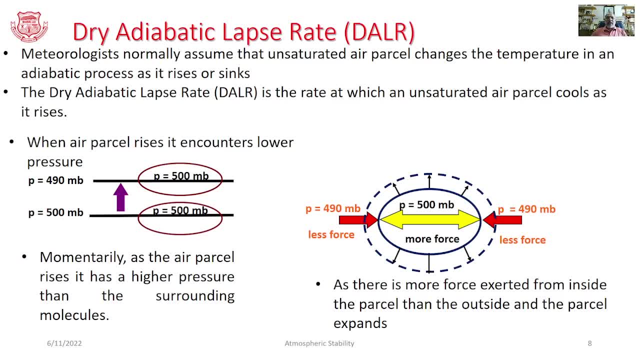 So it is the rate at which unsaturated air parcel cools as it rises. As you see here, When this air parcel rises It encounters the lower pressure. So initially, when at the point of the launching, the pressure is 500 millibars. 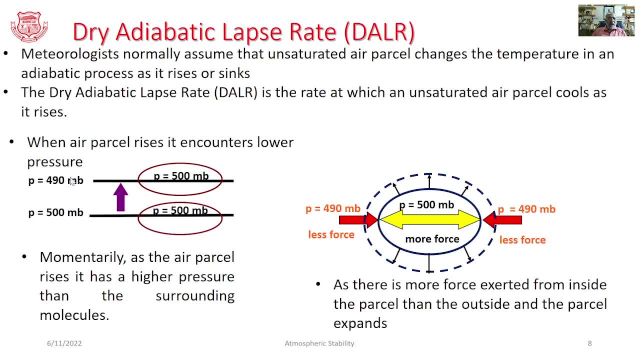 Whereas at it moves up The pressure is 490 millibars. So momentarily, as the air parcel rises, It has the higher pressure as compared to the surrounding pressure, Because here this pressure of the parcel is 500 millibars, Whereas the surrounding pressure is 490 millibars. 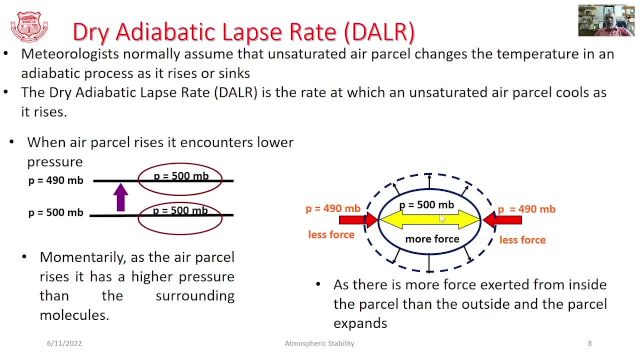 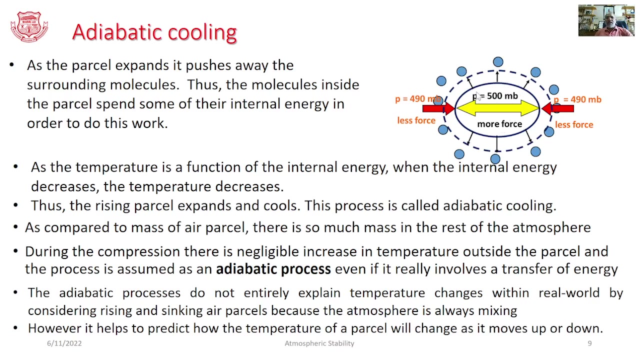 So within the body, As there is a more force exerted from the inside Than the outside, The parcel will simply expand. As this parcel expands, It pushes away the surrounding air molecules, Thus the molecules that are inside this air parcel. 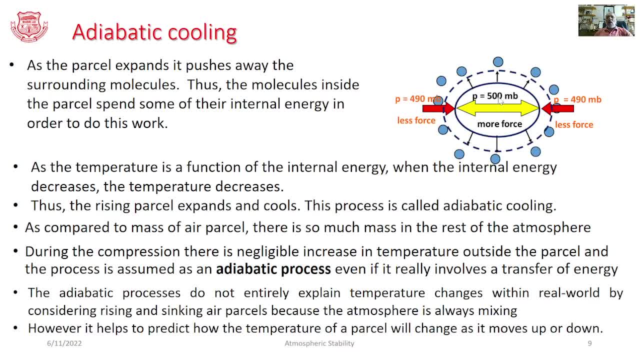 Spends some of this internal energy In order to push away these air molecules, As the temperature is a function of this internal energy. As the internal energy decreases, The temperature also decreases. Thus the rising parcel expands And hence it cools. 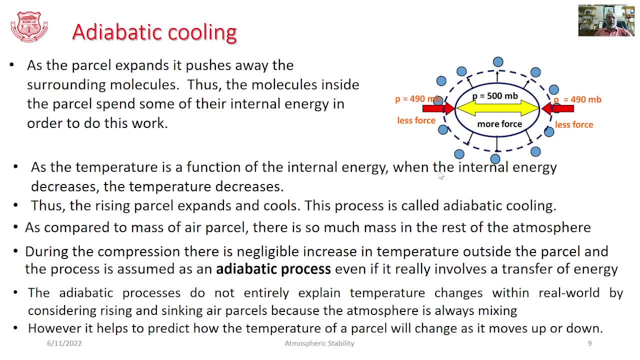 This process is called as adiabatic cooling. As compared to the mass of air parcel, The surrounding mass Is very huge in the rest of the atmosphere. Thus, Though these particular air molecules are pushed away, As this expansion is causing, 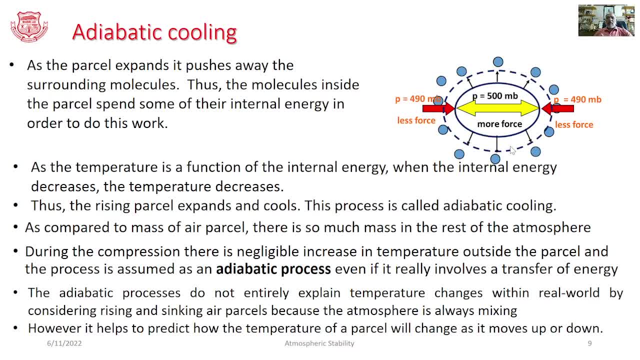 The compression of the rest of the Atmosphere, There is some exchange of the energy. However, As The change in the energy is Very negligible, As it is also associated with the transfer of energy, The process is assumed to be adiabatic. 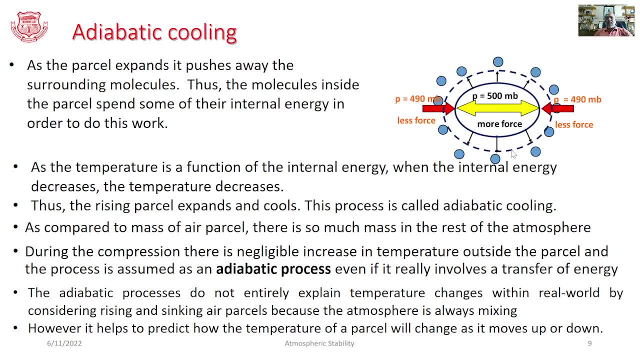 In reality, This process Does not Entirely explain the temperature changes In the real atmosphere, Because There are so many other factors Due to which The atmosphere Is a dynamic, It is not remaining constant. Its nature is not remaining constant. 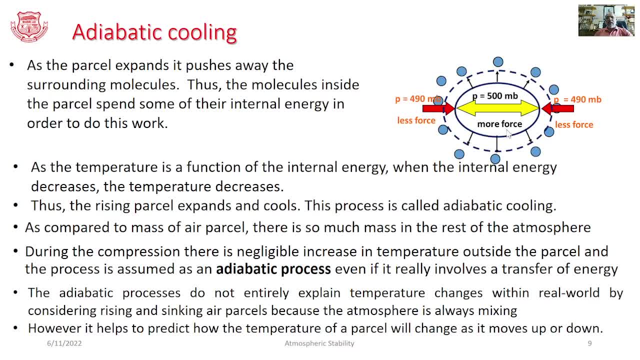 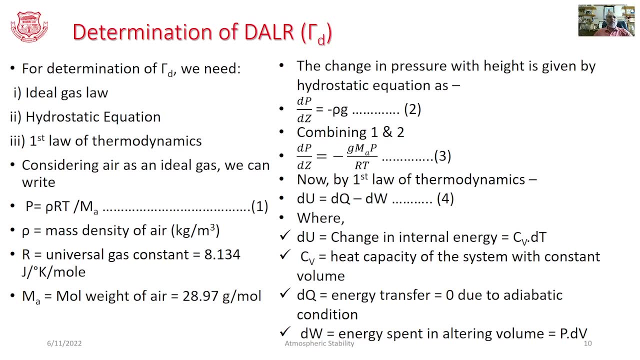 However, This particular terminology we can Use In order to predict How the temperature of the parcel will change As it moves up Or as it comes down In the atmosphere. We can Determine this Dry adiabatic lapse rate. 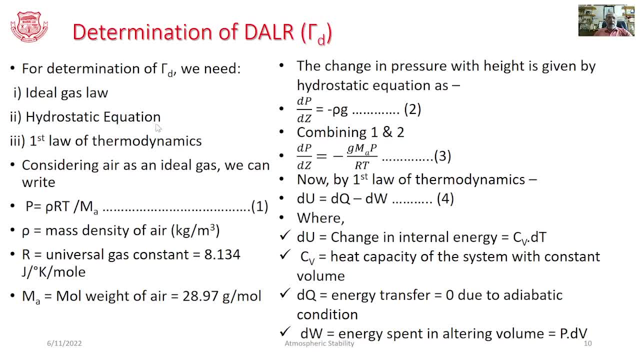 By making use of Ideal gas law, Hydrostatic equation And force law Of Thermodynamics, So considering The air as an Ideal glass, We can Write. Pressure is given as Rho RT, Divided by: 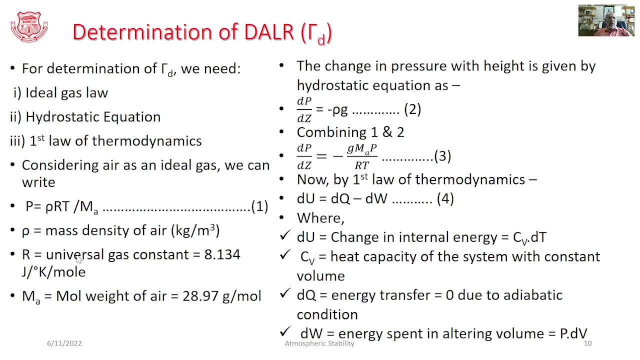 Ma. So this rho is mass density of the air, R is universal gas constant, Ma is the Molecular weight of the air, With the values that are given here. Also, As we consider the Hydrostatic equation, The change in pressure, 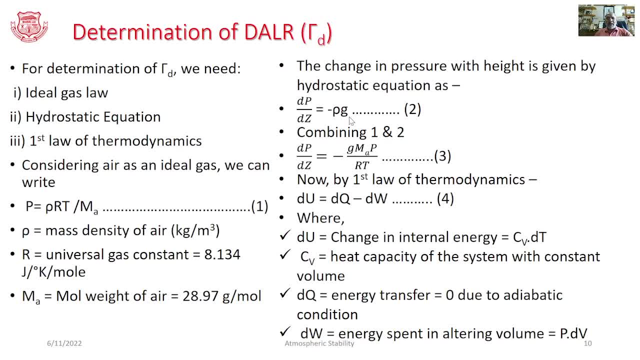 With the height Can be given as: Dp by dz Is equal to Minus rho g. As we compare These two equations, One and two, What we get Is dp by dz Is equal to Minus. 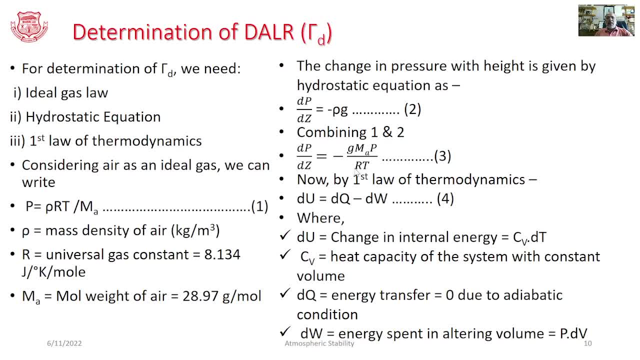 g, M to the base Ap Divided by RT. Also By first law Of the thermodynamics, This du Is equal to Dq Minus dw, Where this du Is Change in internal Energy. 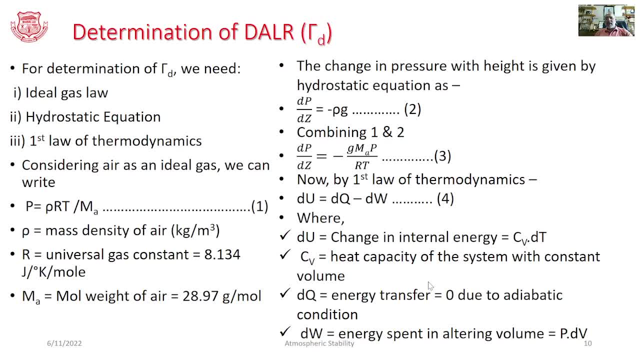 Further given by Cv Times dt. This cv Is the heat capacity Of the system, With constant Values. Dq Is the energy Transfer. For our case, Having the process Adiabatic, This dq. 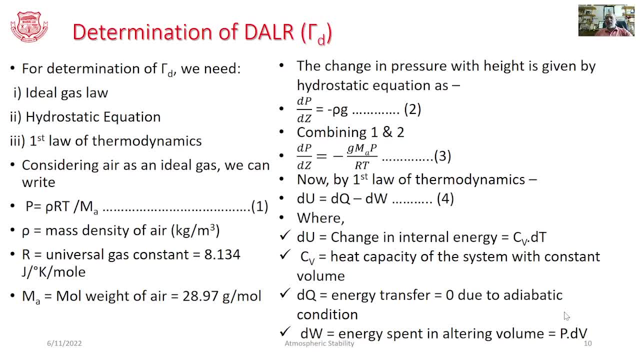 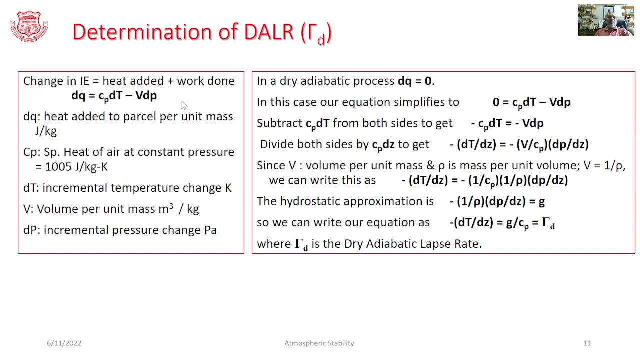 Will be zero And dw Is the energy Which is p times dv. This change In the Internal Energy Is nothing But the Heat Added Plus The energy Associated With the Worktime. 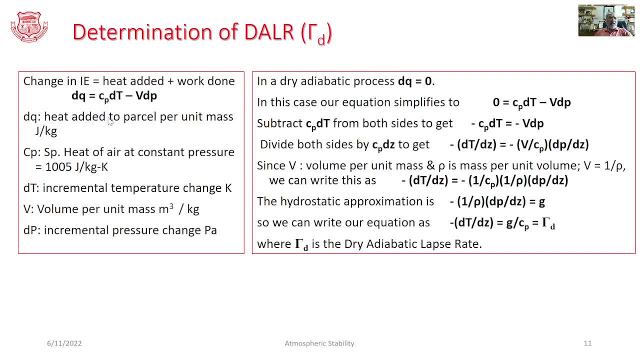 Here This Change In the Internal Energy Is Heat Added To the Parcel Per Unit Mass. This dt Is the Incremental Temperature Change In Degree Kelvins. 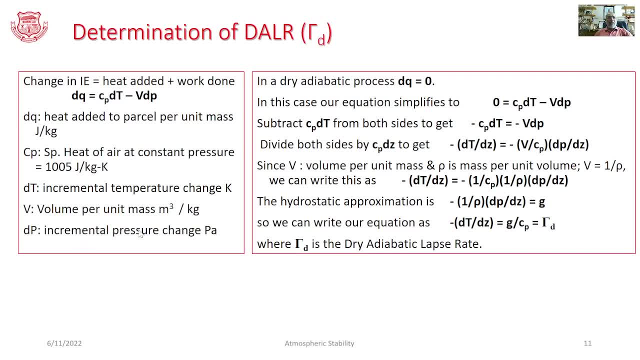 V Is The Value Per Unit Mass Expressed As Meter Q. Per Kg Dp Is The Incremental Pressure Change In Zero Cp Dt Minus. 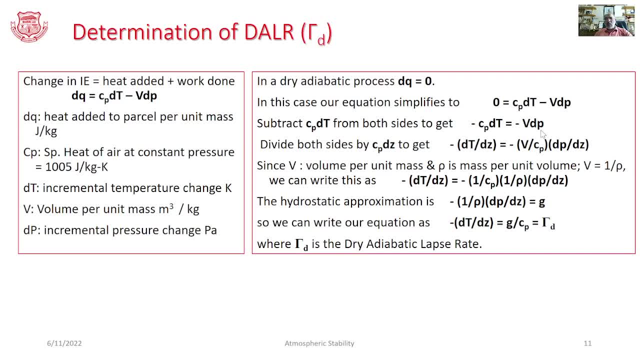 Vdp. Hence Minus Cp Dt Is Equal To Minus Vdp. So As We Divide Both The Sites By Cp Dz, What We Get 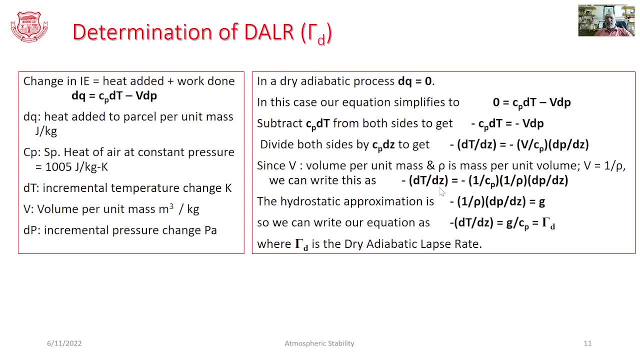 Is Minus One By Rho. Hence The Equation Attains This Form As: Consider The Hydrostatic Approximation Minus One By Rho Into Dp. 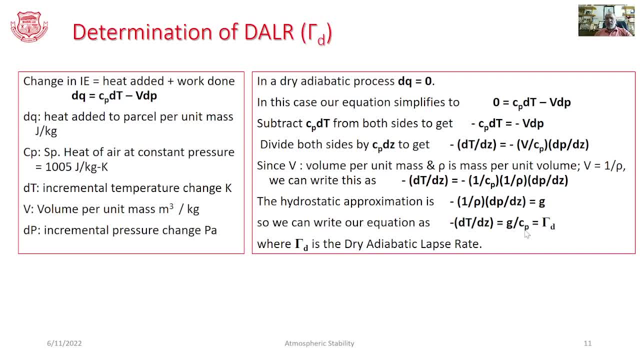 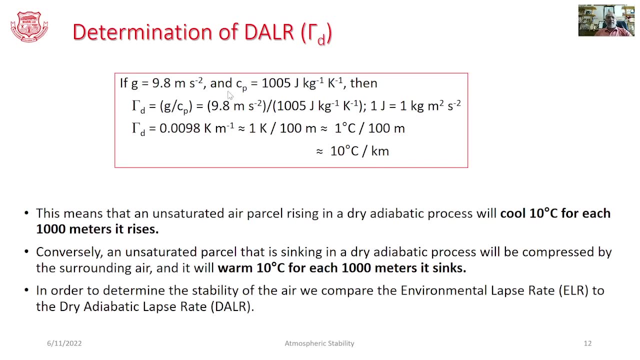 By Dz Is Gravitational Acceleration. Hence The Equation Can Be: Is Dry Adiabatic Lapse Rate, As We Consider The Values G As 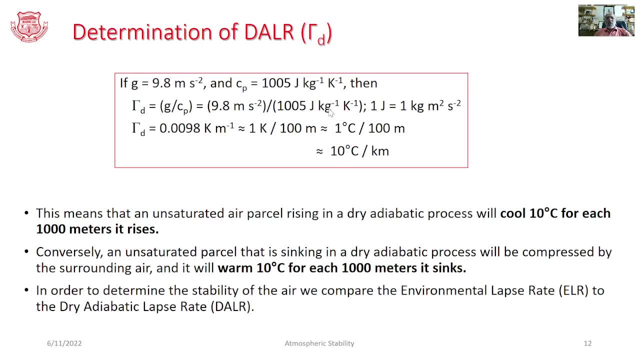 Nine Point Eight Meter Per Second Cp As One Thousand Five Joule Per Kg Per Degree Kelvin Per Meter, So It Is One Kelvin Per. 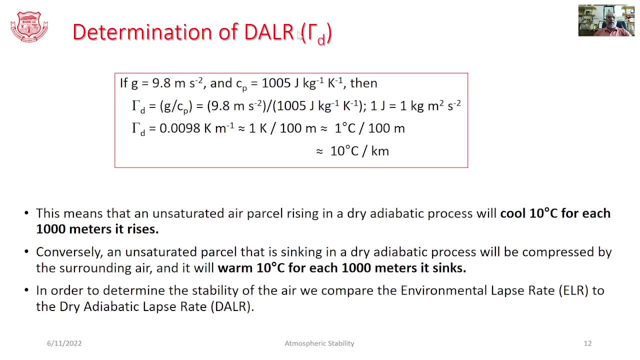 Hundred Meter, Equivalent To One Degree Centigrade Per Hundred Meter. Hence The Dry Adiabatic Lapse Rate Can Be Consider As Ten Degree Centigrade. 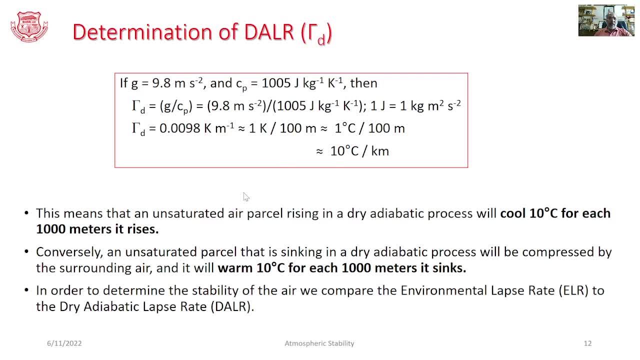 For Each One Thousand Meter As It Rises. Conversely, The Unsaturated Parcel That Is Sinking In The Dry Adiabatic Manor Will Be Compressed. 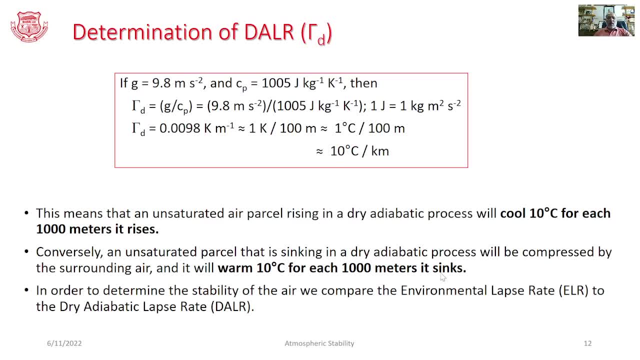 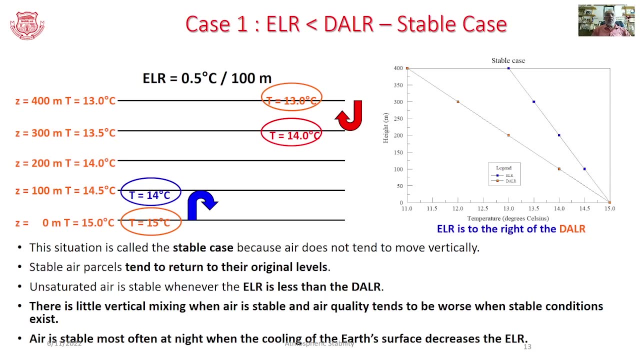 By The Surrounding Air. So To Determine The Stability Of The Air We Have To Compare The Environmental Lapse Rate To The Dry Adiabatic. 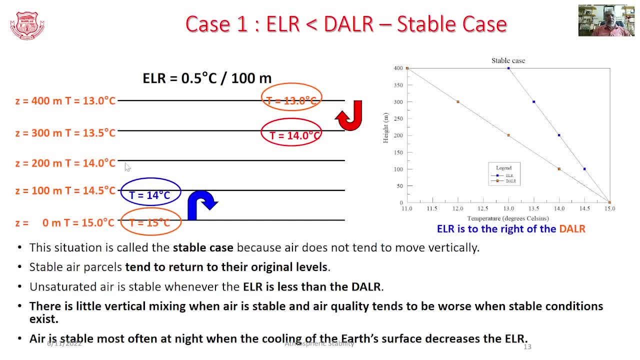 Lapse Rate. So Let's Consider The Various Cases Now. This Environmental Lapse Rate Of Point Five Degree Centigrade Per Hundred Meter. This Is 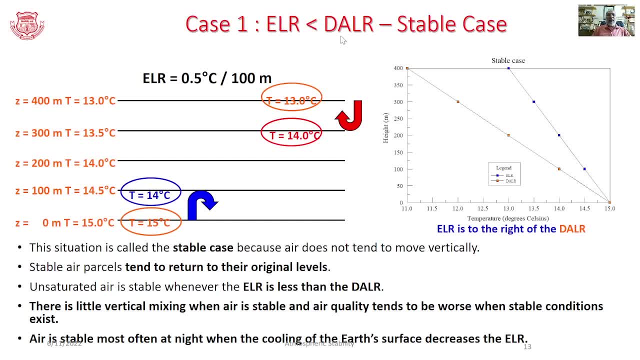 Less Than One Degree Centigrade Per Hundred Meter, Hence This E L R Is Smaller Than Is Point Five Degree Centigrade And Hence. 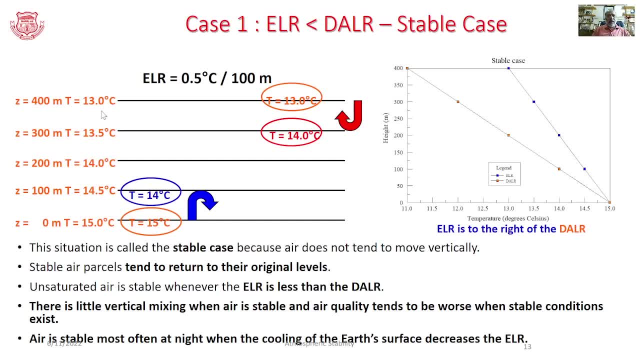 For Every Hundred Meter There Will Be Decreased In The Temperature. At Four Hundred Meter It Will Attend The Atmosphere, Will Attend The Temperature Of 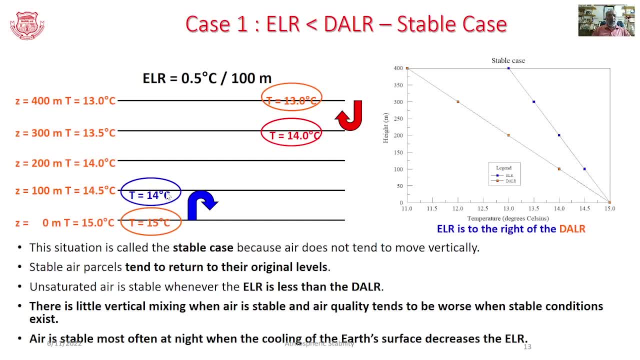 The Degree Centigrade, Because The D? L? R Is Of One Degree Centigrade Per Hundred Meter. Hence, At Hundred Meter, The Air Parcel Has. 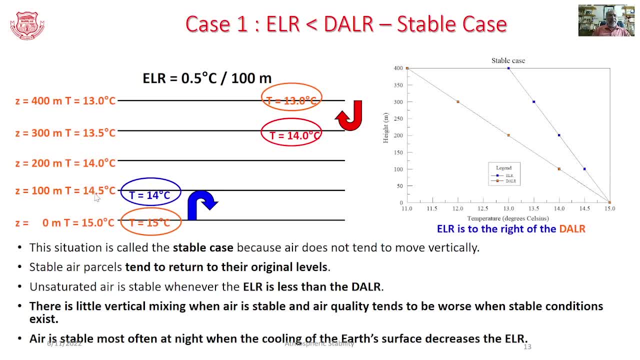 Got Temperature Is Of Forty Five Degree Centigrade, As The Air Parcel Has Got Lesser Temperature As Compared To The Surrounding It Has To. 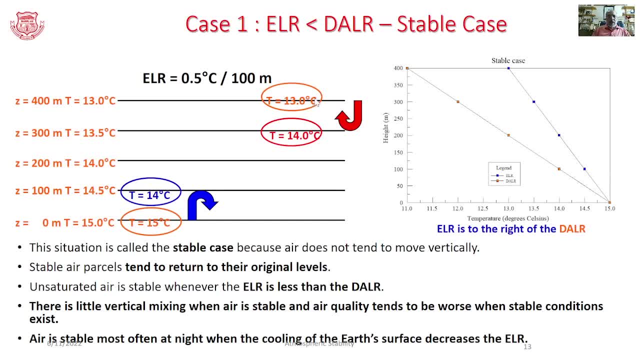 Sink Down, And Hence It Is Stable. As It Sinks Through The Hundred Meter, It Will Be Attaining The Temperature Of Forty Degree Centigrade. 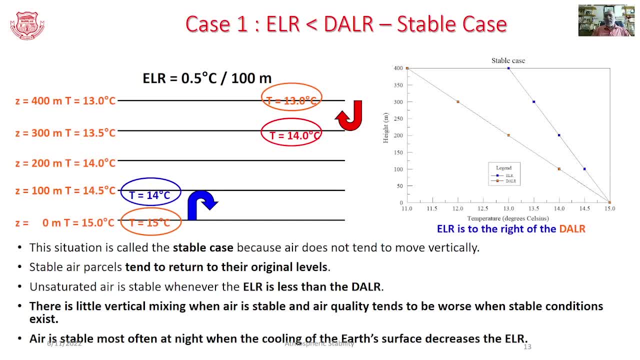 As It Is Compared To The Surrounding, The Temperature Is Higher, That The Air Is On The Right Side Of The Air. Also, It Means 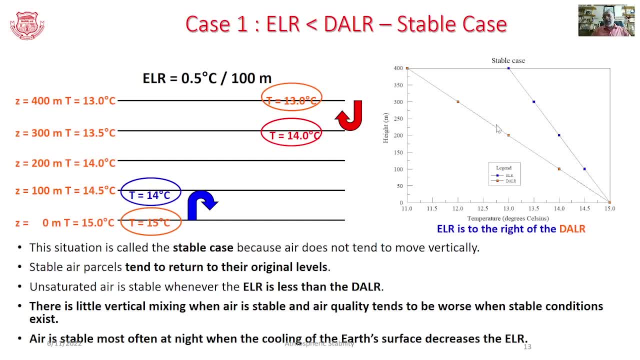 The Air Is On The Left Side Of Air, Hence The Condition Is Sub Adiabatic. So This Is Stable. So This Case Is Stable. 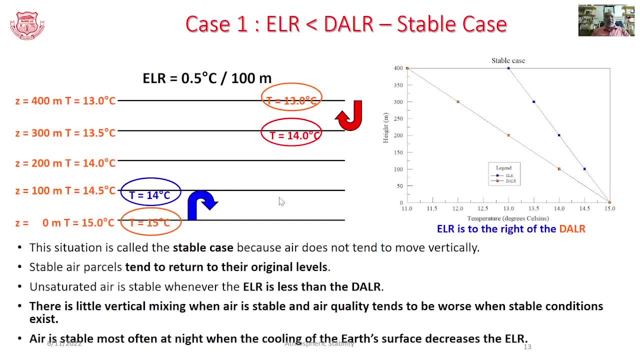 Because There Is Not Vertical Mixing As We Discuss Here, The Stable Air Parcel- Tend To Return To Their Original Level Conditions. Most Of The 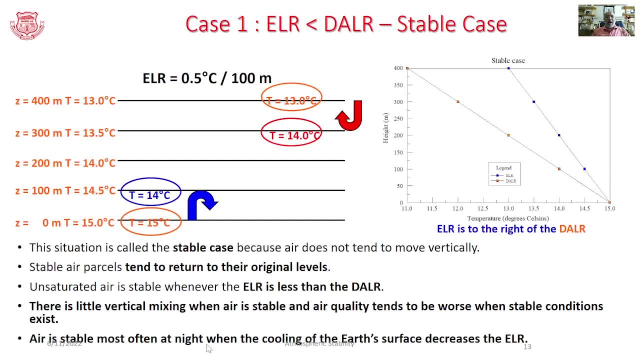 Times. This Situation Will Be Prevailing During The Night Time, As The Cooling Of The Earth Surface Has Got Direct Impact Over This Are Associated. 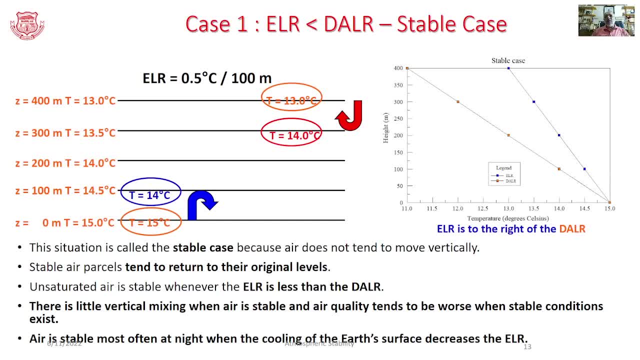 With The Stable Cases- And That Are Further- That Have In Fact Occurred Over The Night Time Or Early Mornings. One More Effect Associated With 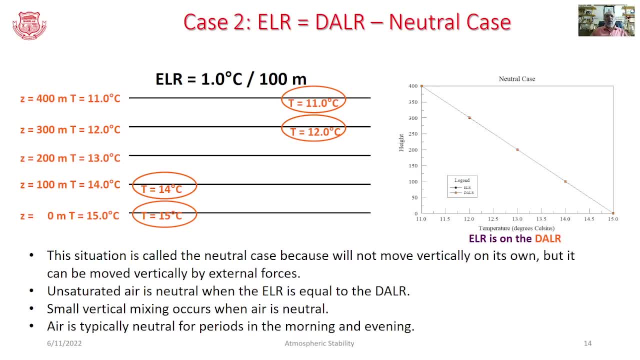 Disasters Will Be Prevailing Here. For Case Two, The L? R And D? L? R Is Same. Again, We Are Considering L? R Of One. 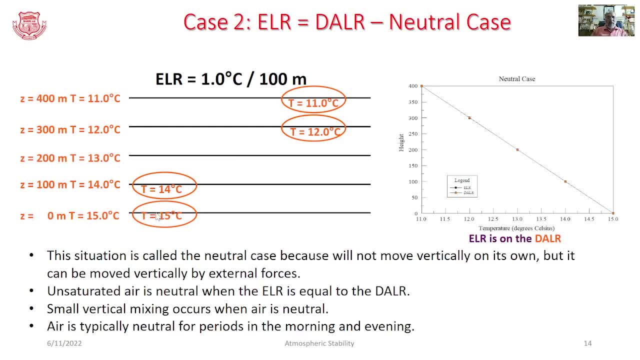 Degree Centigrade Per Hundred Meters, Which Is Same As Got The Temperature Of Fifteen Degrees Centigrade As It Moves To The Hundred Meters. 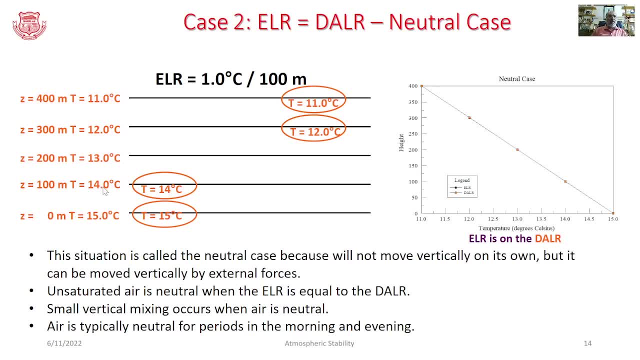 It Will Be Getting Cold Adiabatically, And Hence It Will Attend The Temperature Of This Twelve Degrees Centigrade, Because It Will Be Warmer. 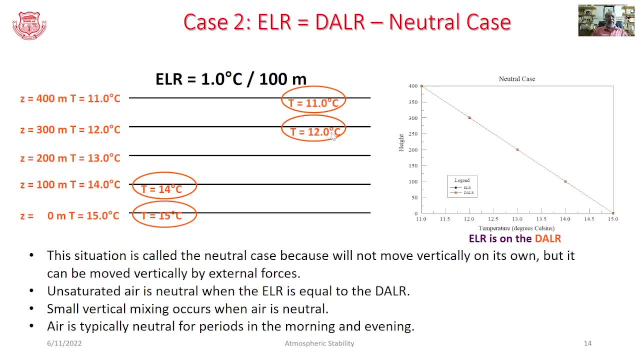 This Temperature Is The Same As That Of The Surrounding Temperature, And Hence It Will Be Remaining At That Altitude While R Profile Dry Adiabatically. 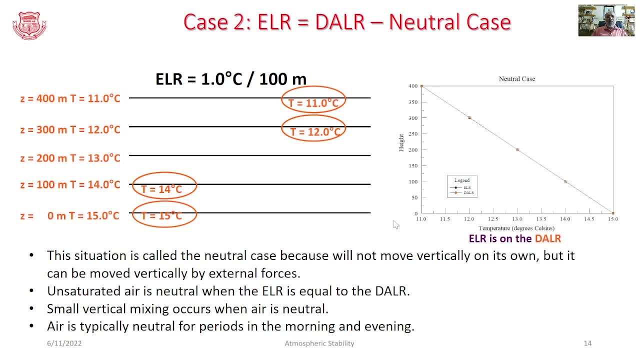 Lapse, Like Profile Are Overlapping Each Other, So This Situation Is Called Neutral, Because There Won't Be Any Vertical Mixing On The. According To 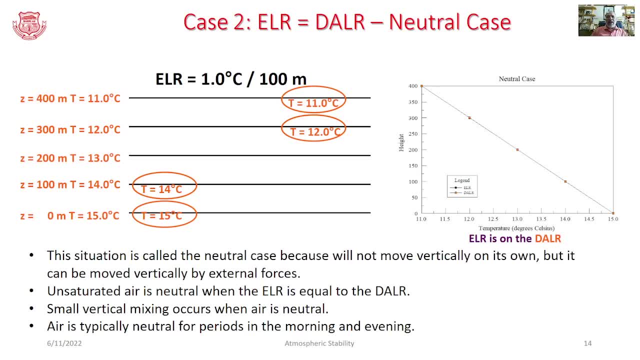 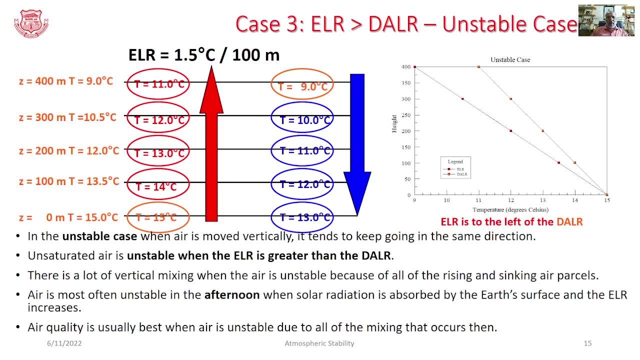 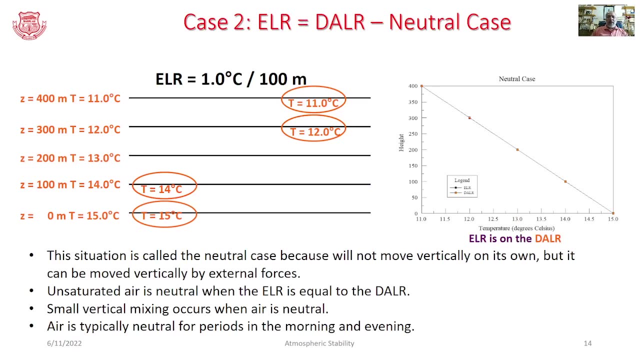 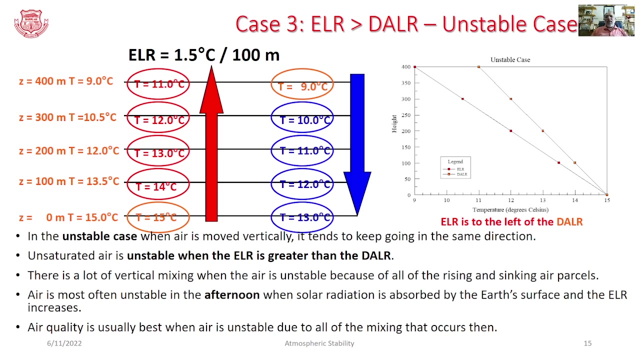 occurs when ELR and DLR are equal. there is a very small vertical mixing. also, the air is typically neutral in early morning period and evening period. case 3 is showing ELR to be greater than DLR. so the way you see this ELR is to. 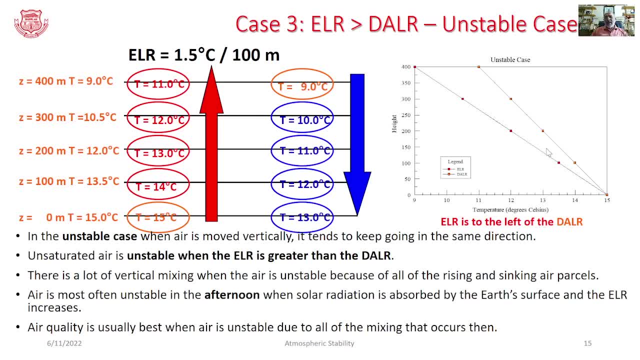 the left of the DLR. DLR is on the right side. hence the condition is treated to be super adiabatic and it leads to unstable case. as you see here, this ELR is 1.5 degree centigrade per hundred meters. here this: 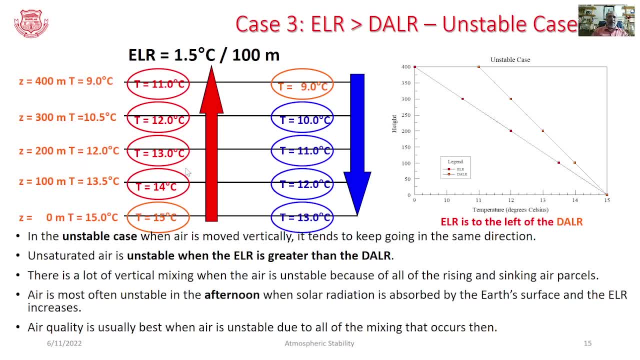 lapse is shown on the left side at the ground level, as the air parcel has got the same temperature as that of the surrounding. however, as it is lifted up as it moves through hundred meters vertically adiabatically, so the adiabatic process will lead to how that parcel temperature of the 14 degree 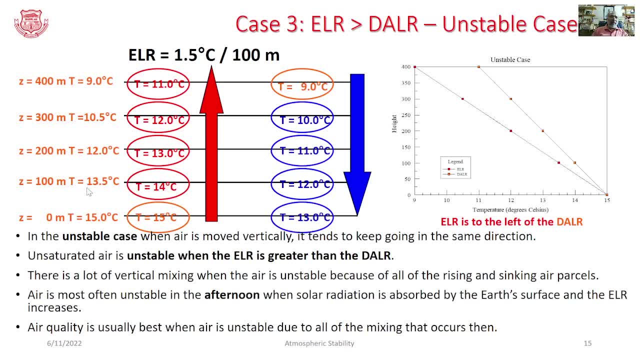 centigrade, which is more as compared to the surrounding temperature, and hence the parcel will keep on rising and this rising will be continued till it has the same temperature, till it will attain the same temperature as that of the surrounding temperature. hence the case is treated to be unstable. similar effect is considered as for 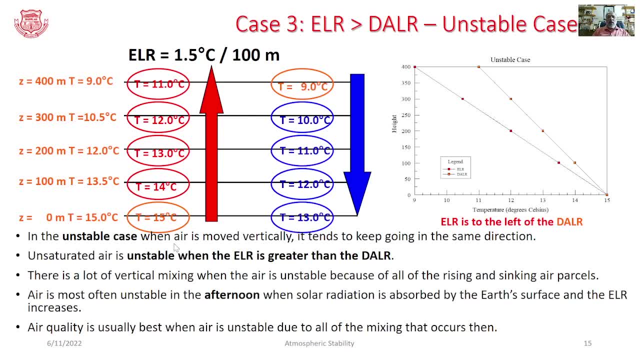 the sinking of the sample is concerned. so in the unstable case, when the air is moved vertically, it tends to keep on going in the same direction. unsaturated air is unstable. when this ALR is greater than DLR, there is a lot of vertical mixing. when the air is unstable because of the rising as well as the sinking of 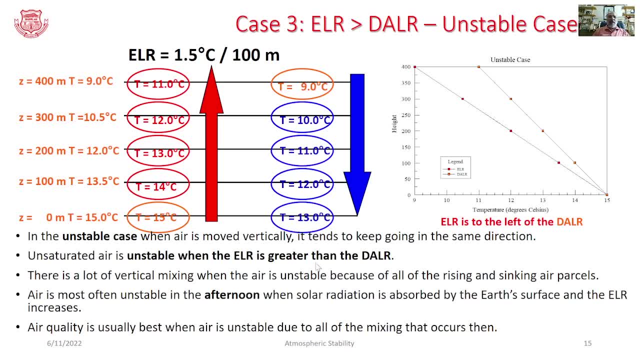 the air parcel, and this condition is mostly observed when the solar insulation is high, especially during the solar radiation is high, especially during this upturn, as there is a considerable mixing associated with the unstable case. the pollutant, once emitted, will be getting transported at the high altitudes as it has the higher temperature, hence here. 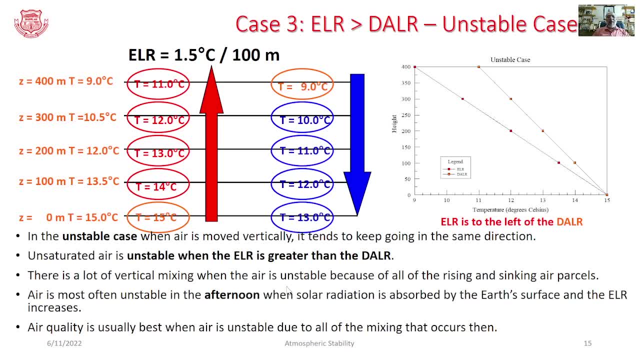 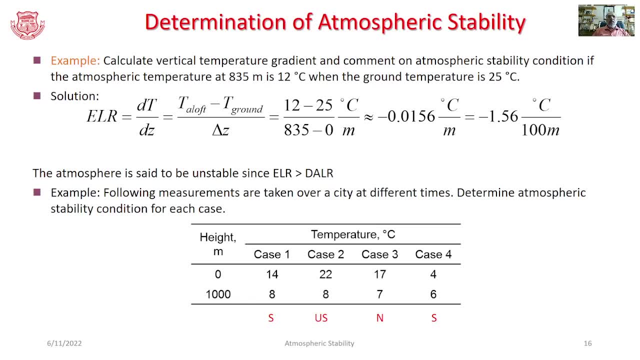 the air quality will be comparatively quite good in unstable cases. as we have the data collected at the various weather service stations, or climate crazy. air quality will be comparatively good in unstable cases. as we have the data collected at the various weather service stations or climate monitoring stations, it can be used in order to determine this atmospheric stability. so here say: 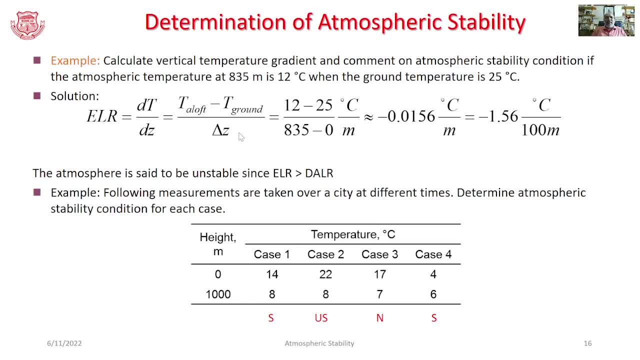 the allow temperature is of 12 degrees centigrade, whereas the ground level temperature is of 25 degrees centigrade, and if the change in the height is of 835 meters, there will be EL are of 0.0156 degree centigrade, so this will be minus 1.56. 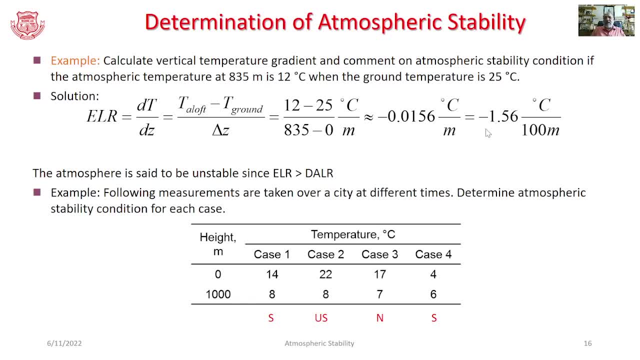 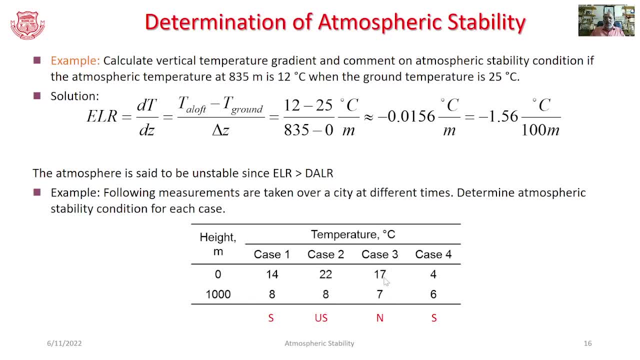 and this is unstable condition here- ELR being equal to DLR, the case will be neutral. this is just reverse the case. the atmosphere will be highly stable because it is not allowing the vertical rising of the pollutant, because the temperature at the upper altitude is higher. 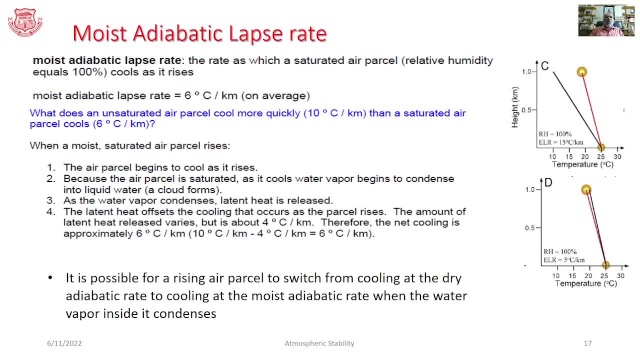 Now, the third category of this lapse rate is moist adiabatic lapse rate. we consider the hormonal lapse rate, we consider air sample to be dry and hence the dry adiabatic lapse rate. This moist adiabatic lapse rate is associated with the saturated air parcel, that is, when the relative humidity equals the 100%. 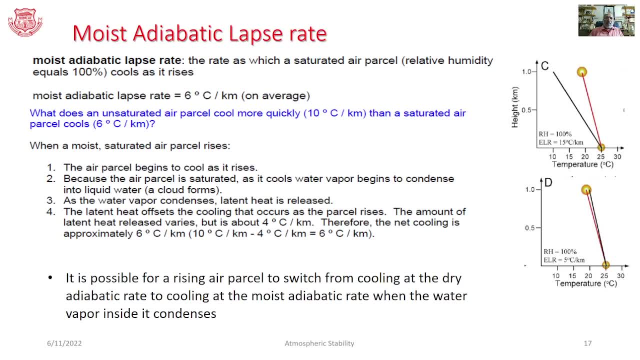 This moist adiabatic lapse rate is not remaining same because the dew point varies with the altitude. However, the moist adiabatic lapse rate can be considered to be 6 degree centigrade per kilometer on average. When we consider the saturated air parcel, that is rising. 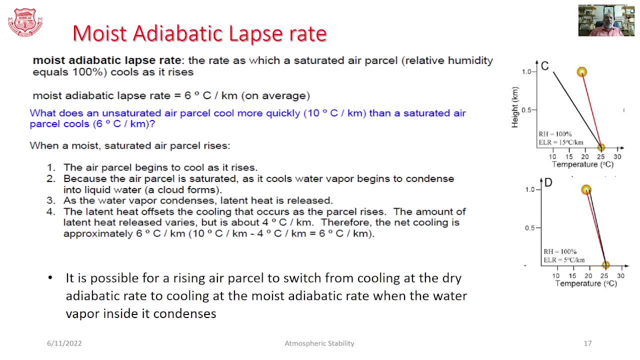 as it rises, it begins to cool. As the air parcel is saturated and as it cools, the water vapor it has will be condensed into the liquid, and hence there will be formation of the clouds. As the water vapor condenses, the latent heat is released, and this latent heat offsets the cooling. 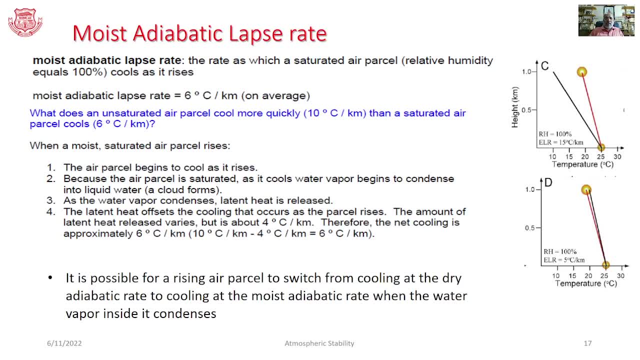 that occurs as the parcel rises. The amount of the latent heat released varies, but it can be taken as 4 degree centigrade per kilometer and hence the net cooling is considered to be 6 degree centigrade per kilometer. The water vapor is considered to be 6 degree centigrade per kilometer. 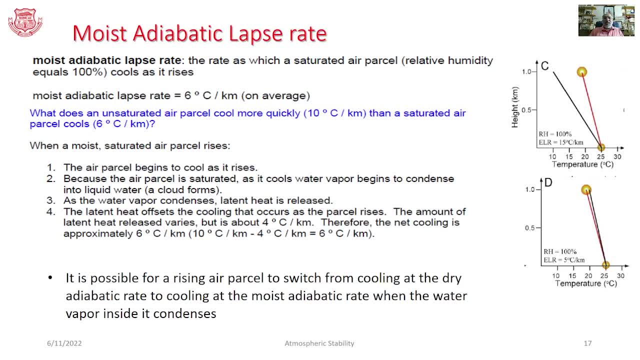 It is possible for rising air parcel to switch from cooling at the dry adiabatic rate to cooling at the moist adiabatic rate as the water vapor inside that parcel condenses. In line with the discussion that we had here, this red line is showing the moist adiabatic lapse rate, whereas that black line is showing 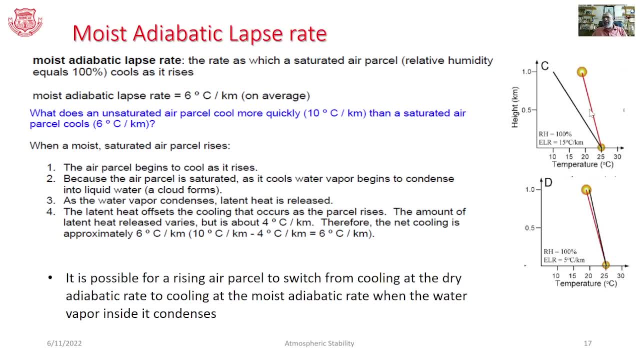 the ELR. As we consider this MALR moist adiabatic lapse rate to be 6 degree centigrade and the ELR 15 degree centigrade. having this ELR greater than MALR, now the condition will lead to unstable, Whereas as we consider the environmental lapse with 5 degree. 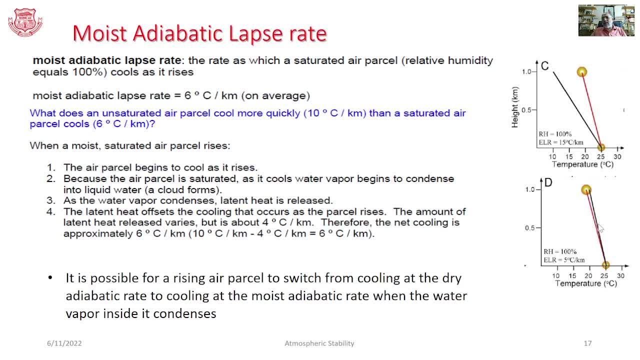 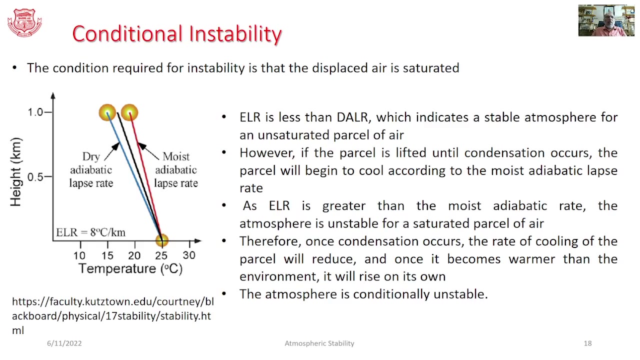 centigrade per kilometer and the environment and the moist adiabatic lapse rate of the 6 degree centigrade per kilometer, there is not much difference. The condition will be approximately neutral As we consider the dry adiabatic lapse rate or moist adiabatic lapse rate having the value 10 degree. 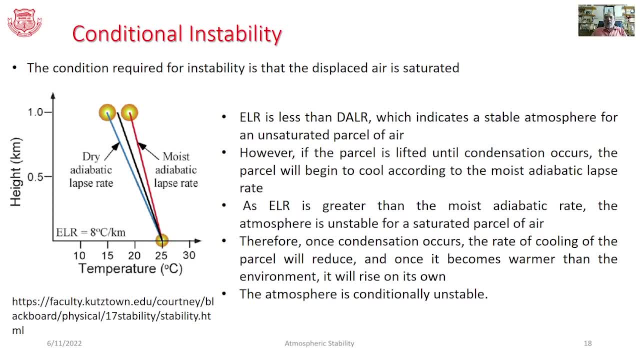 centigrade per kilometer, or 6 degree centigrade per kilometer. in case we consider the environmental, in case we consider the saturated air pass, there can be certain intermediate condition. say, for example, here the ELR is 8 degree centigrade per kilometer, so the ELR is lying. 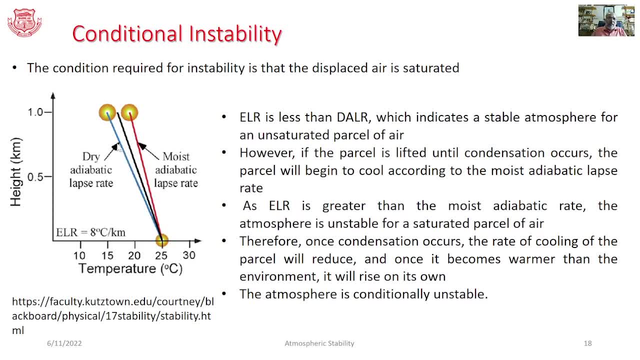 in between the dry, the line representing the dry adiabatic lapse rate and moist adiabatic lapse rate. as we compare this ELR, it is less as compared to dry adiabatic lapse rate. hence this will indicate the stable atmosphere as far as dry parcel is concerned. 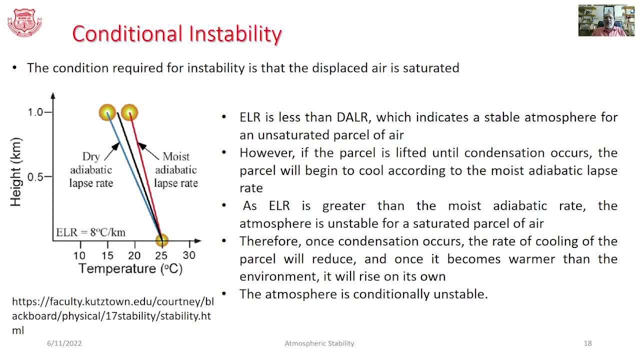 however, as the parcel is lifted up until the condensation of the water vapor occurs, the parcel will begin to cool according to the moist adiabatic lapse rate. so as we compare the further cooling with the moist adiabatic lapse rate, here the 8 degree centigrade ELR is greater than 6 degree centigrade per kilometer moist adiabatic. 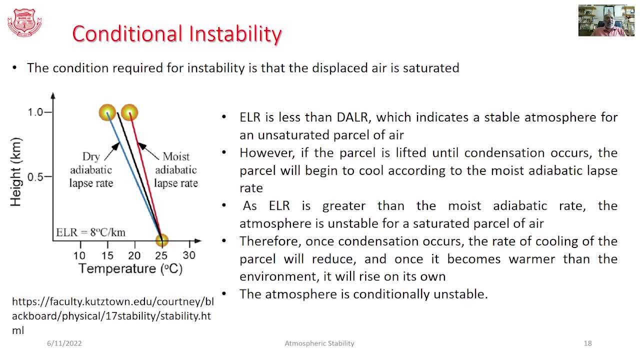 rate and hence, as far as this situation is concerned, the atmosphere is unstable for saturated parcel of the air. so for the dry sample it will lead to stable atmosphere. for saturated sample it will lead to unstable condition. hence, once the condensation occurs, the rate of the cooling of the parcel will reduce. 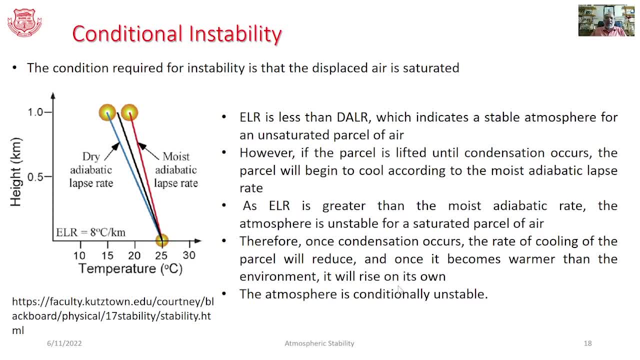 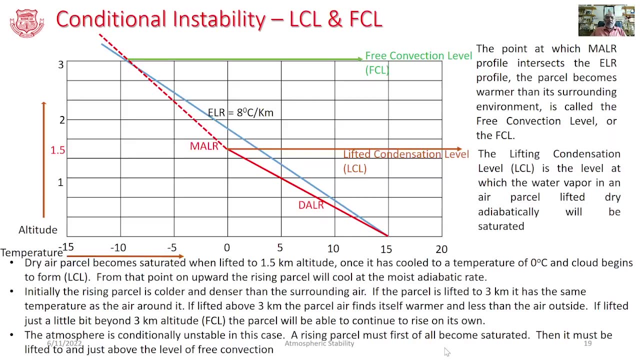 and once it becomes warmer than the environment, it will rise on its own. this is conditional and hence the atmosphere is treated to be conditionally unstable. this situation is further elaborated. we have considered this ELR to be 8 degree centigrade per kilometer. 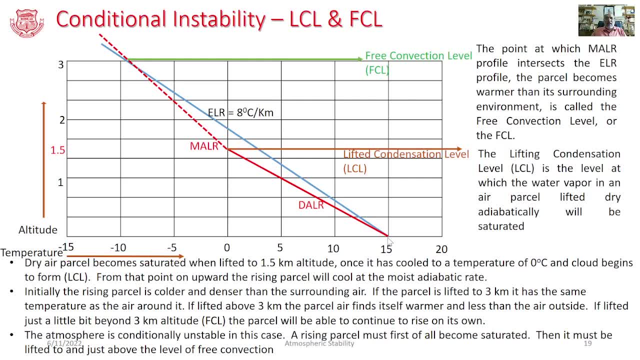 at the ground level, the temperature is of 15 degree centigrade. as one attains the height of the 3 kilometer, there will be temperature of minus 9 degree centigrade. as you see here, initially the air parcel which is emitted at the ground level and as it is treated to be dry, as it. 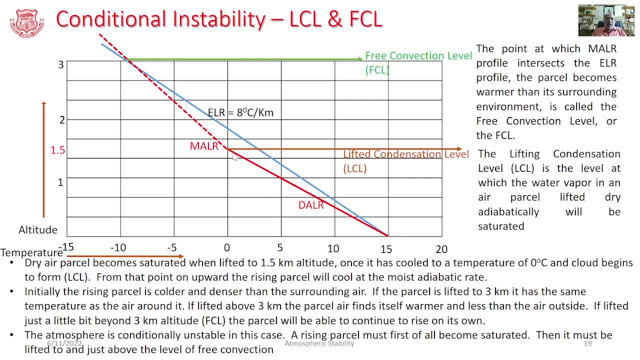 is lifted up at height of 1.5 kilometer, it will be attaining the temperature of the 0 degree centigrade and hence there will be the formation of the cloud. this point onwards, if the parcel is lifted up, the parcel has to follow the. 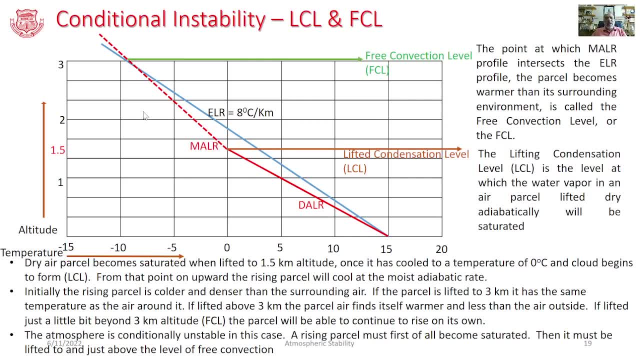 moist adiabatic collapse rate. so accordingly, as it moves up further 1.5 kilometer it will also attain the temperature of the minus 9 degree centigrade. so at 3 kilometers height the air parcel will be having the same temperature as that of the surrounding temperature. 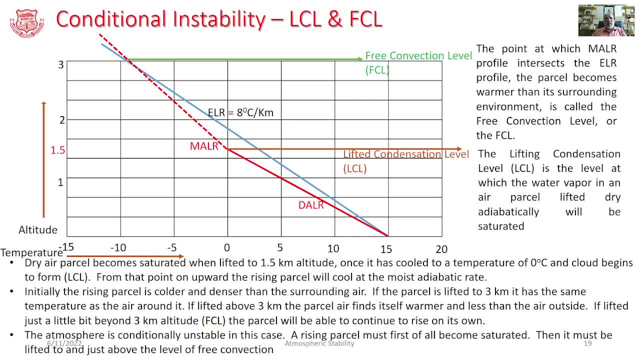 however, somehow, if this particular parcel is further moved up, it will be warmer as compared to the surrounding temperature and it will keep on rising on its own. so this is conditionally unstable case. but in order to have these conditions, this rising parcel must be first of all saturated, and then it must be lifted. 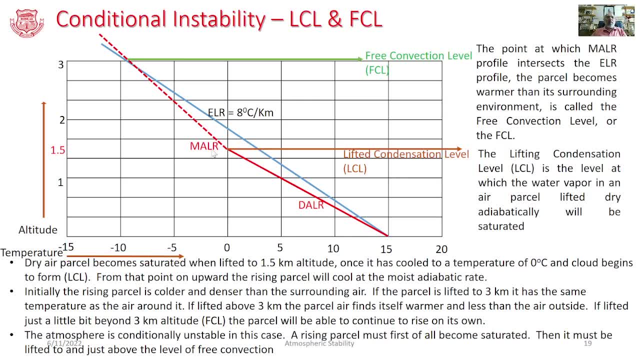 to and just above the level of precorrection. here, as you see, the point at which the temperature attained is 0 degree centigrade. it is treated to be lifting condensation level, which is a level at which the water vapor in the air parcel which is was lifted adiabatically and which 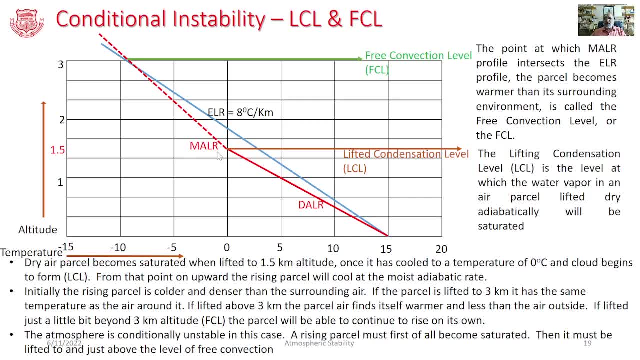 was dry, will be fully saturated, whereas the point at which it attains the same temperature as that of the surrounding, which is preconvection level. it is the point at which this moist adiabatic lapse rate intersect with the environment lapse rate and the parcel becomes warmer. 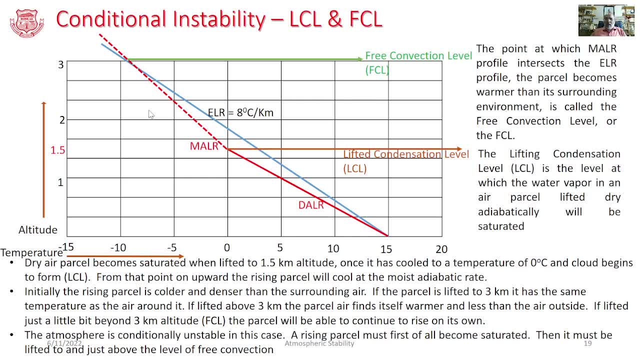 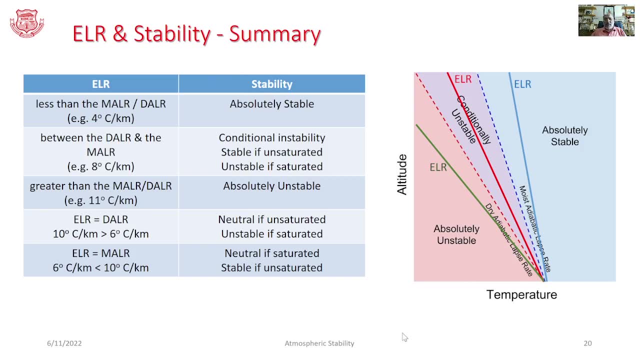 than the surrounding environment which is associated with the conditional instability. So the entire discussion that we had is summarized here. The condition could be absolutely stable. As you see here, environmental lapse rate is on the right side of moist adiabatic lapse rate. 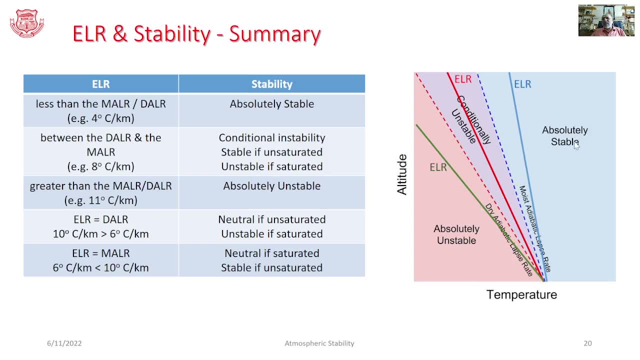 as well as dry adiabatic lapse rate. Hence it is absolutely stable Here. the adiabatic lapse rate- environmental lapse rate- is on the left side of moist adiabatic lapse rate, as well as dry adiabatic lapse rate. 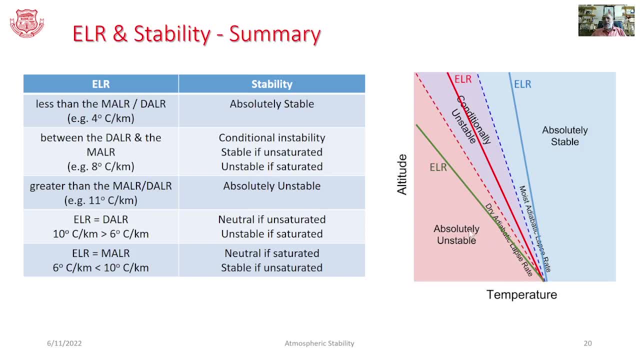 Hence the atmosphere is absolutely unstable, Whereas in between moist adiabatic lapse rate and dry adiabatic lapse rate, if the ELR is low, there will be conditionally unstable case. Same thing with dry adiabatic lapse rate. 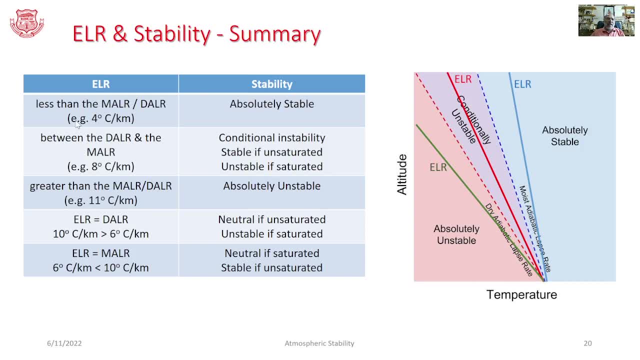 If the ELR is less than MALR as well as DALR, say for example, 4 degrees centigrade per kilometer, the condition will be absolutely stable Here if the ELR is lying in between DALR and the MALR. 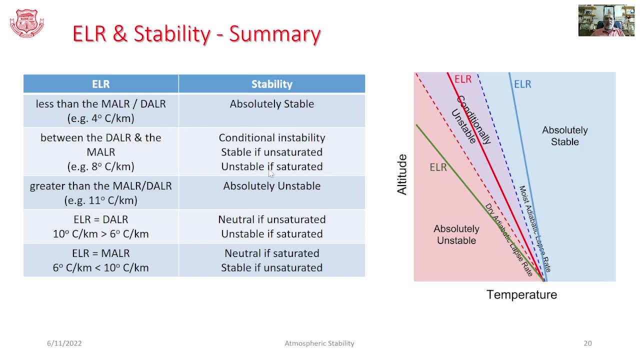 there will be conditional instability. If we consider the unsaturated air parcel, the situation will be stable. If we consider the saturated air sample, it will be unstable. If the ELR is greater than both MALR and DALR, there will be absolutely unstable case. 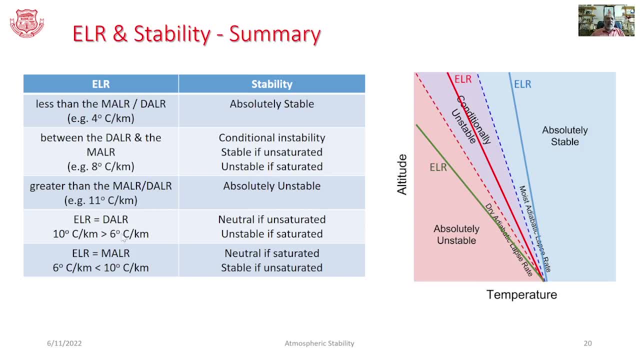 Say, for example, 11 degrees centigrade per kilometer. If both are equal, it will be neutral case. Still, if we consider this ELR's ELR to be 10 degree centigrade per kilometer and if it is greater than 6 degree centigrade, 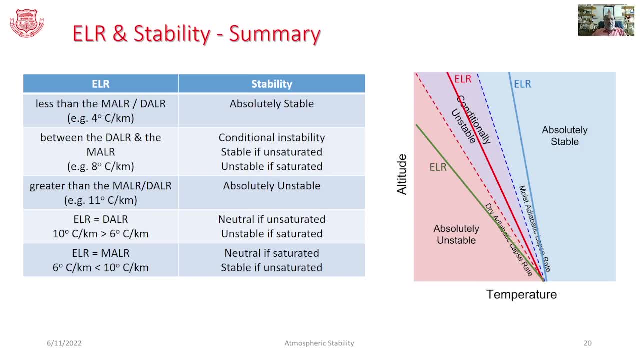 per kilometer. the situation can be considered as neutral if unsaturated, whereas unstable if saturated. if ELR is equal to moist adiabatic lapse rate And if we consider the air parcel to be saturated, it will lead to neutral stability, whereas as we consider this ELR to be 6 degree centigrade per kilometer, which is less than 10 degree,